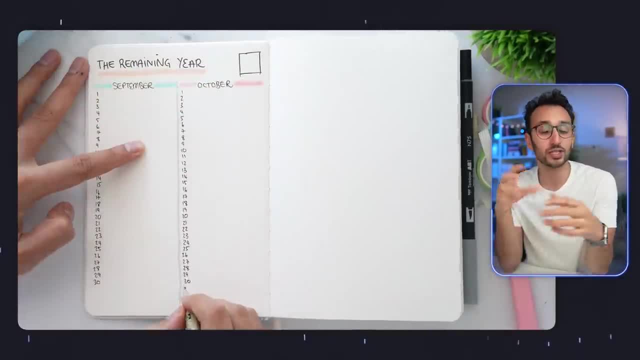 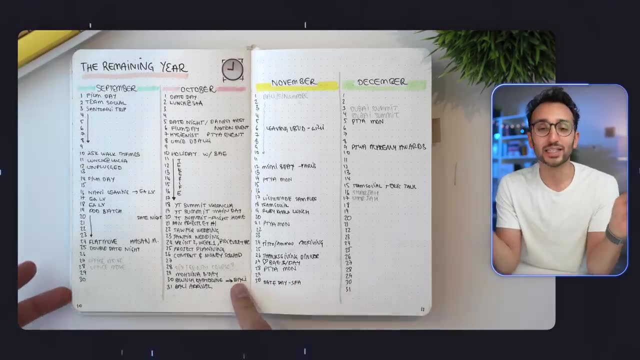 show the different months and then one to 31 down the side that show you the different dates, And so what you end up with is these 366 blocks. Now, when I did this, when I did the bullet journal technique, this immediately gave me incredible insight and clarity into what the rest of my year. 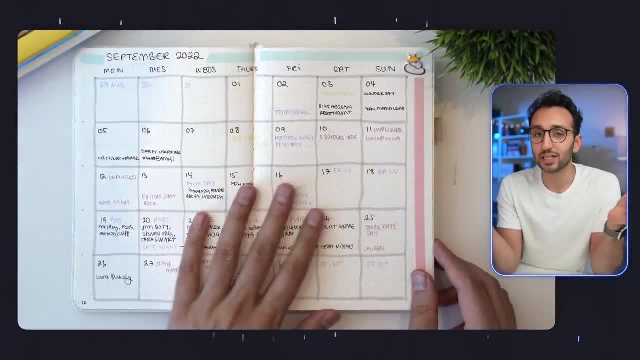 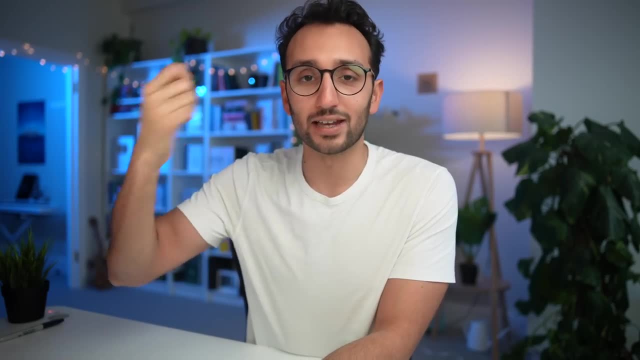 was going to look like, Because this is not really a view that we see particularly often. If, for example, you use Google Calendar or something, you tend to be stuck in the weekly view or in the monthly view, And even if you have like a physical annual calendar, you tend to flip the pages And so 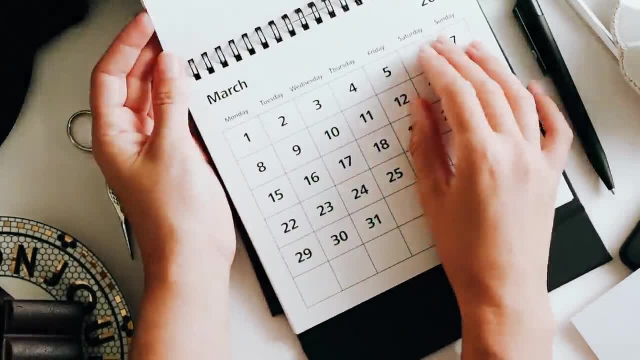 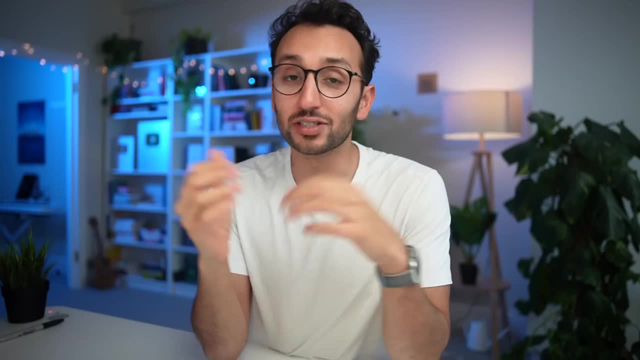 you never really see your entire year just laid out on a single page or two pages. So in January of this year I decided I wanted to have a more digital way of having this kind of view in my life, And so I decided to just make a Google Sheet out of it. I think these days it's too easy to default. 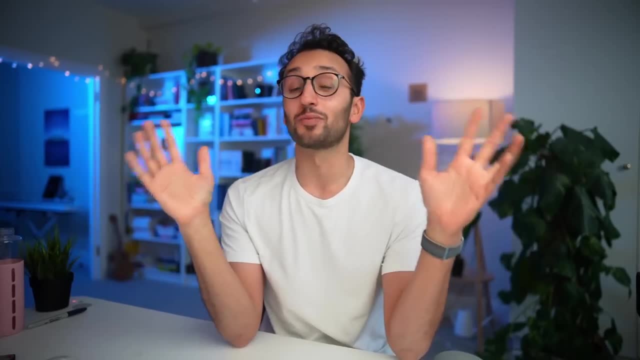 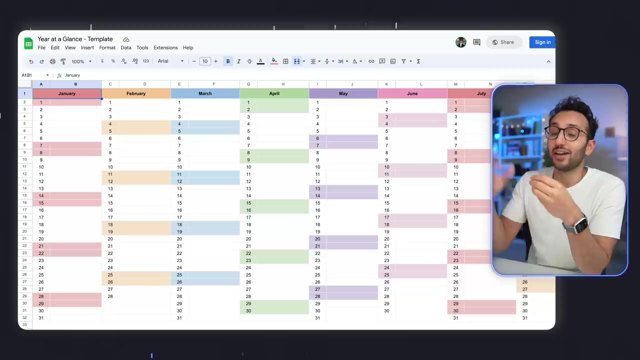 to fancy apps and like, oh, what's the latest thing here? But I thought you know what A spreadsheet just does the job totally fine. And so I literally just went through on Google Sheets and I created one of these year at a glance- templates, And this is what- the blank version. 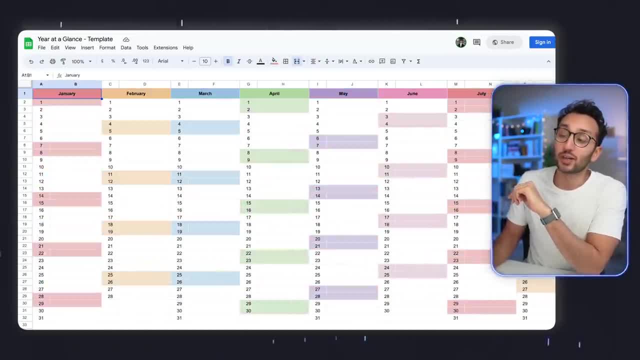 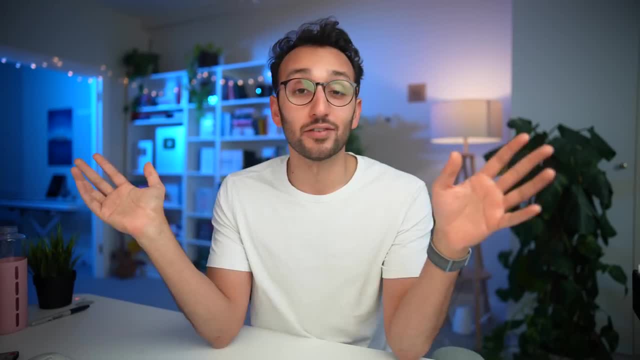 of this looks like. So, as you can see, we've got the months down the top, We have color coded the months in like pretty colors and we've got the weekends color coded as well, And this is the template that you can download. Just hit the link in the video description. It's completely free and 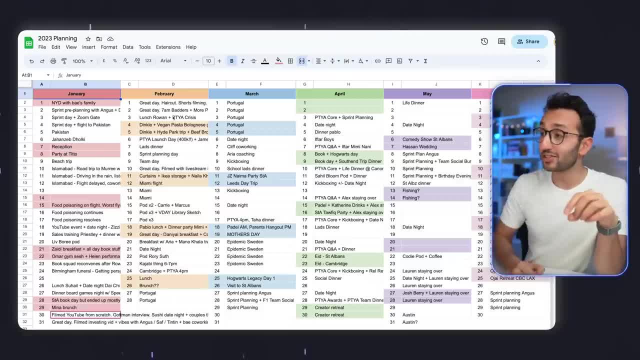 you can duplicate this into your own Google Sheet account. You would really like to, And this is what my version of this actually looks like, And I use this in two specific ways to manage my time. Firstly, it's really helpful for zooming out. 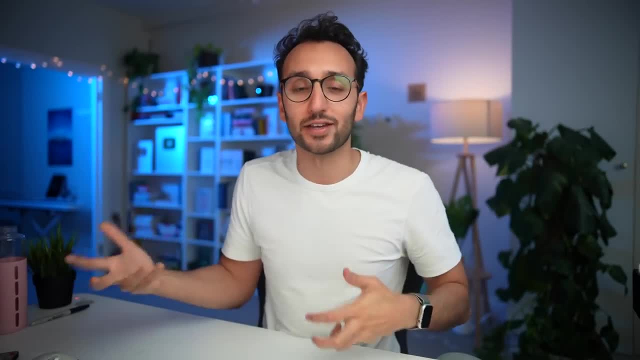 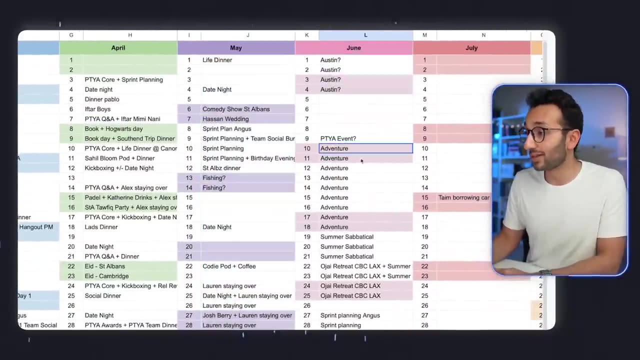 and getting a bird's eye view of my entire year so I can use it to plan my life. I'm filming this video, for example, in April, but I already know that this is the stuff that's kind of going on in May And in June I'm going to Austin for a bit And then I've got this block of time to go. 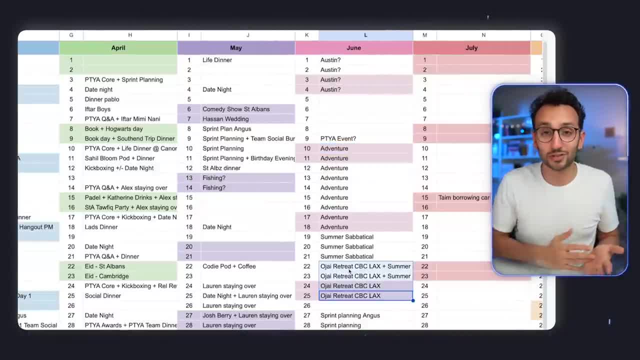 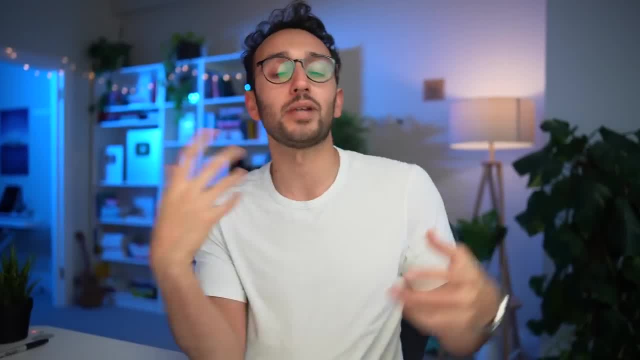 on an adventure with some friends And then I'm going on a retreat to LA later in June And this is so helpful to get an idea of A- where things are, and B. it then allows me to plan things like weekend group trips with friends or being able to plan holidays in advance, so I can block out the 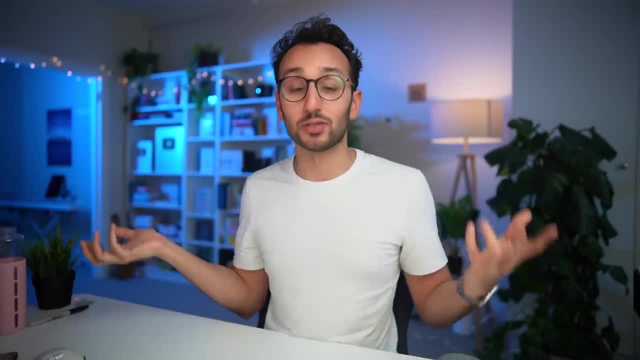 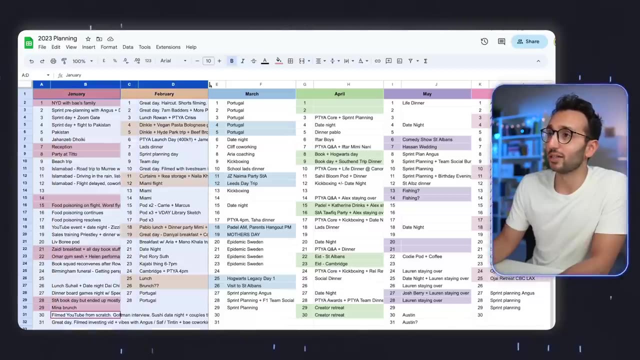 time. I then reflect those changes in my actual Google calendar, so the team knows exactly what's going on in my life, And I found this to be a ridiculously effective way of managing my time on a macro scale And to make this easier to deal with. what you can do is when the months are gone. 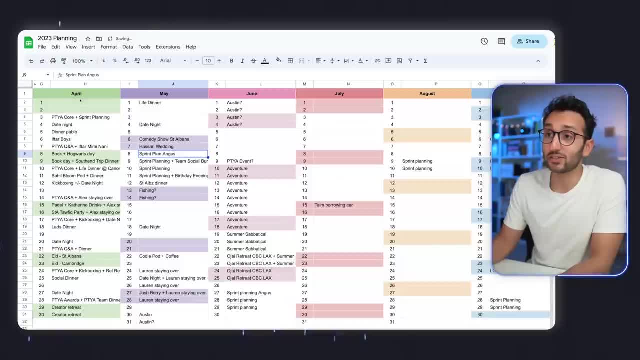 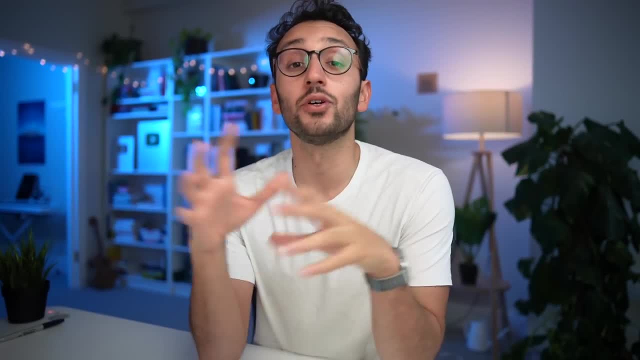 you can just right click, you can hide those columns, And now it's just way easier to see exactly what's going on in a given month and then what's going on for the rest of the year. So that's how I manage my time on the level of the whole year. Let's now move on to the level. 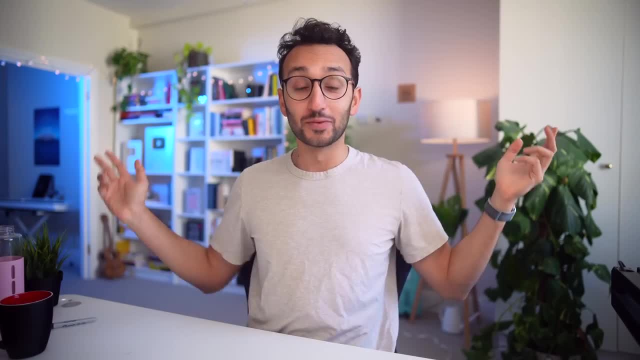 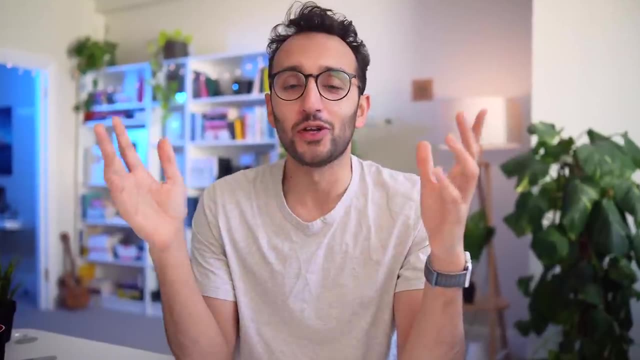 of a single week, But I've got to go somewhere right now. Be right back. Good morning, It's a new day and we are talking about component number two, which is all about ideal week planning. Now here's the context behind this. So, essentially, we all have these goals and 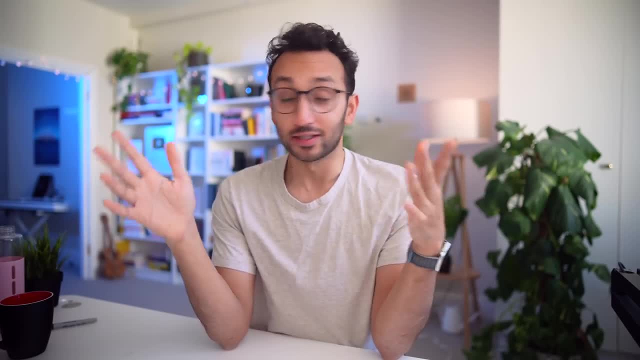 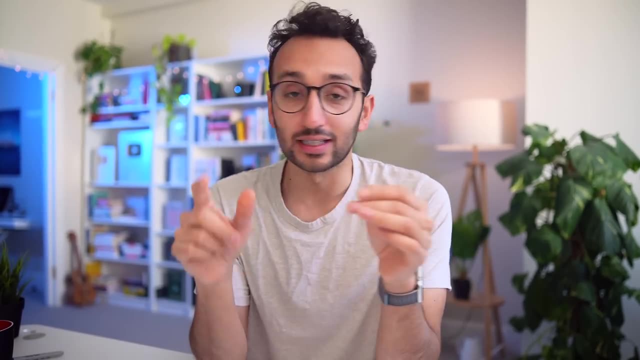 plans and stuff that we want to get done Now. please don't cancel me for saying this, but there are literally just 24 hours in a day and we all have to decide how we're going to make the most use of that time. If, for example, you have three personal assistants and five private chefs and 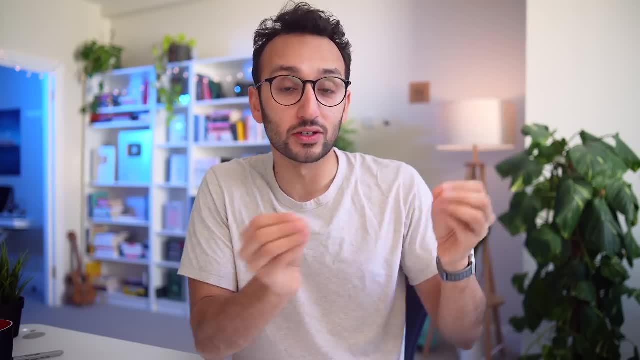 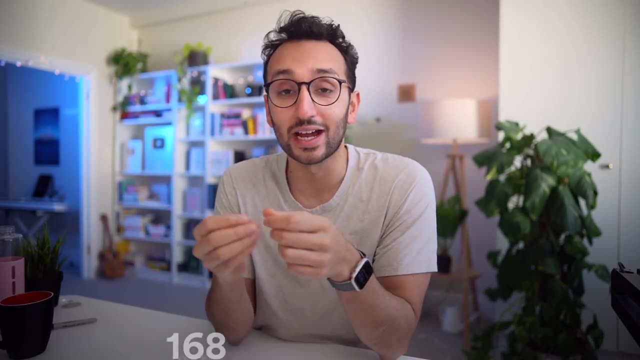 stuff, then obviously you will have more of those 24 hours that are free to do things that you want to do rather than do things like laundry and cooking and cleaning and stuff. But fundamentally those 24 hours or 168 hours a week are basically the same for everyone And, assuming you're 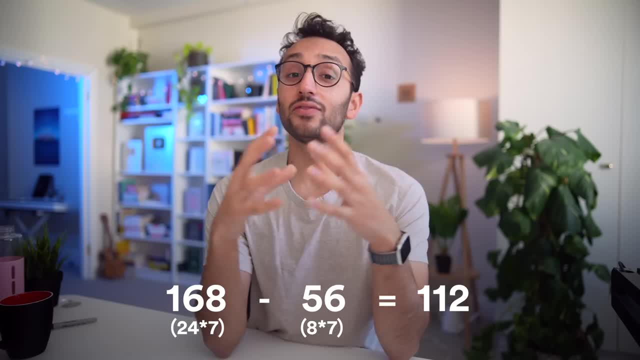 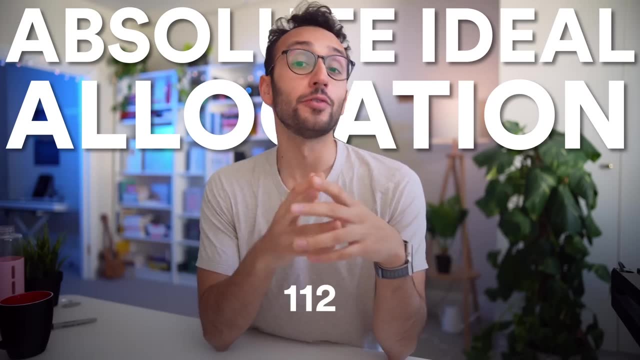 sleeping for eight hours every night. we all basically have 112 hours in a given week that we can play with, And the point of component number two is that we want to define the ideal week, ie our absolute ideal allocation of those 112 hours per week, And this is a method I've been 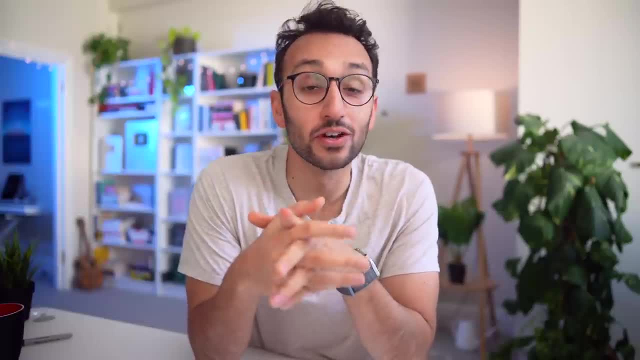 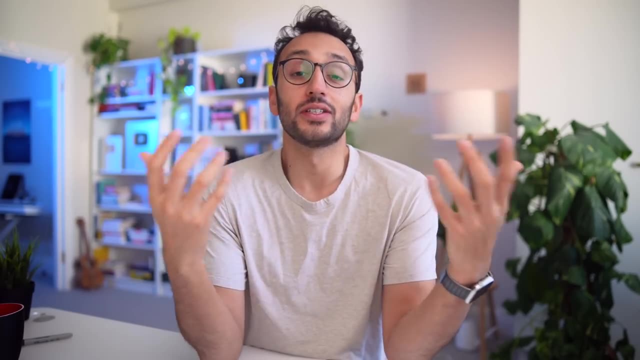 using for the last eight months or so, ever since I started working with my CEO coach, Eric Partaker- And Eric has worked with a couple of hundred CEOs of really high growth companies and me- And this is one of the methods that he asks all of his clients to do, And apparently it's a method. 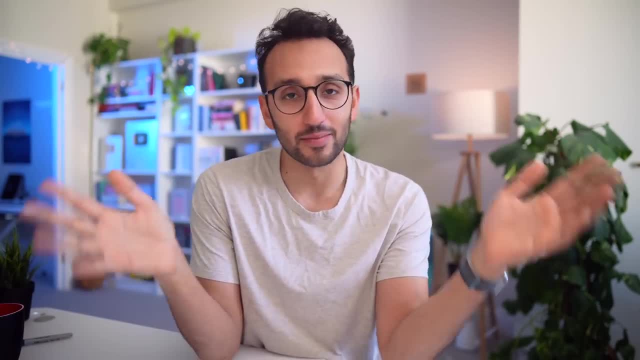 that always gets some results, And it's certainly gotten me a lot of results over the last eight months. And so, instead of you having to pay several thousand dollars an hour for Eric's time, I'm just going to teach you the method straight up, And it's actually fairly straightforward to. 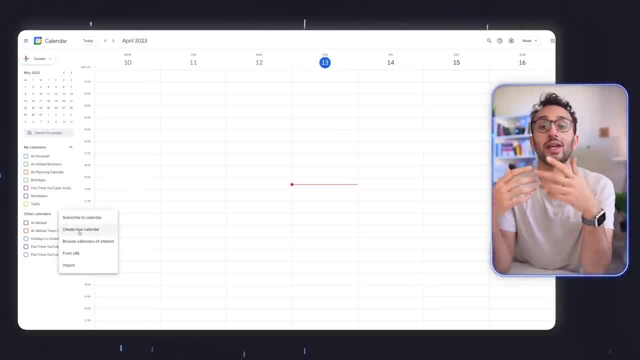 do. All it involves is going on Google calendar and it involves creating a new calendar so that you've got a completely fresh slate where you can do your ideal week planning- Cool. So I've now created Ali's ideal week And now you can see it's shown up in my Google calendar right here. 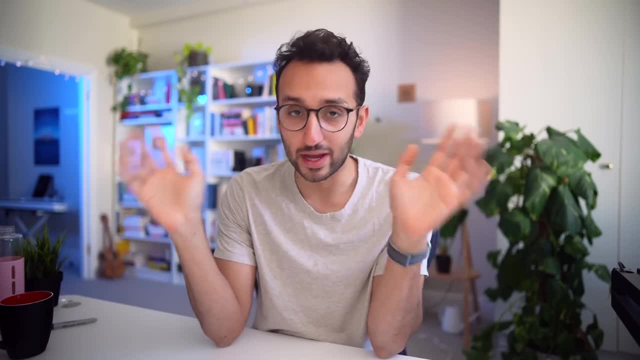 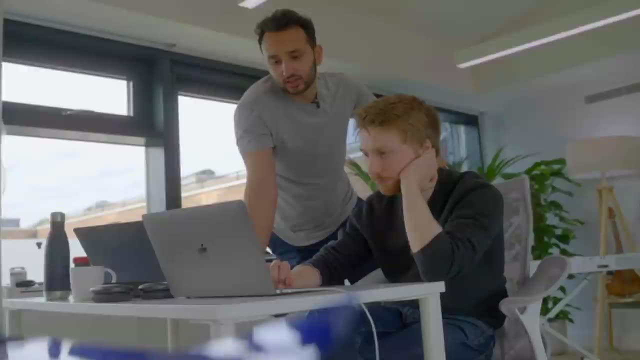 and this is completely free. Everyone can use Google calendar. You don't have to pay a penny, ever at all. Now, at the moment, my life is a little bit of a mess because of the YouTuber academy happening and because of all the book stuff going on and all the meetings with the 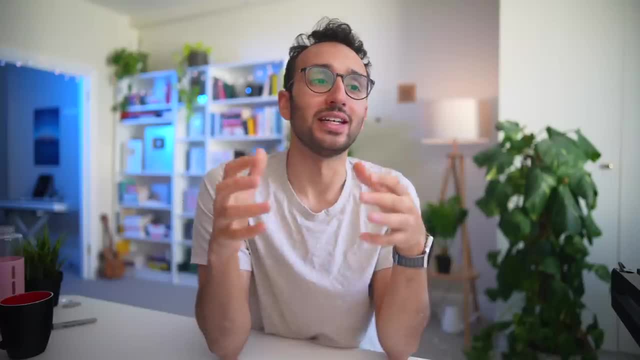 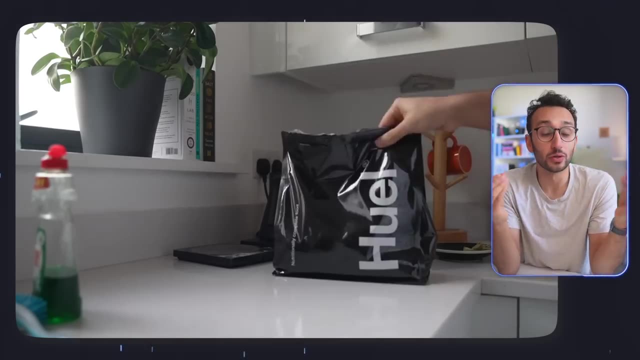 editors and agents and all of that fun stuff, And so what can often happen is that I actually don't have that ideal lunch hour in which I'd like to cook a healthy lunch, And so instead, a product that I've been finding a lot of use of is, in fact, Huel, who are very kindly sponsoring this video. 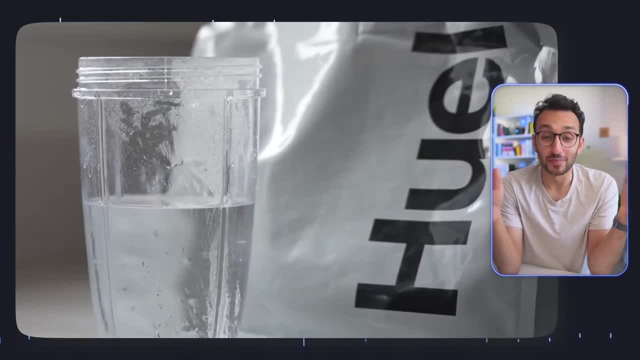 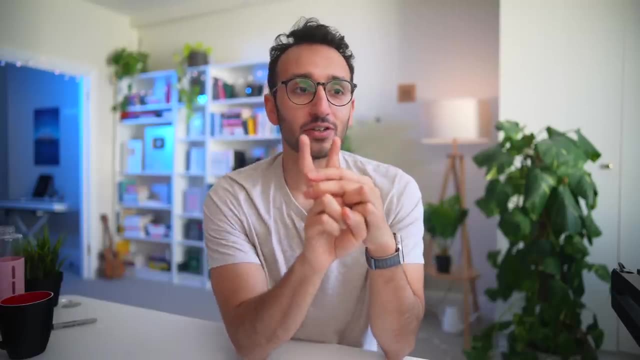 Now I've actually been a paying customer of Huel since 2017 and since my penultimate year of medical school And actually when I first started this YouTube channel six years ago. I've been taking Huel fairly regularly And there's broadly two types of Huel that I really enjoy. The first one: 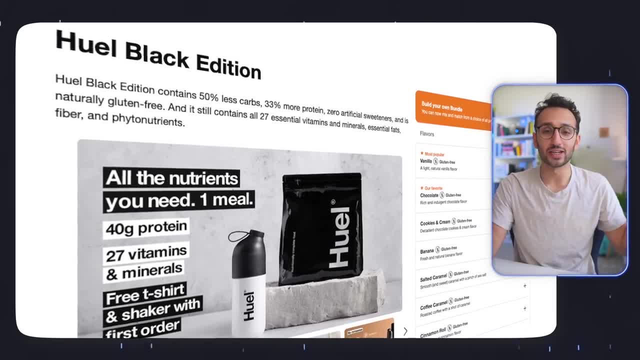 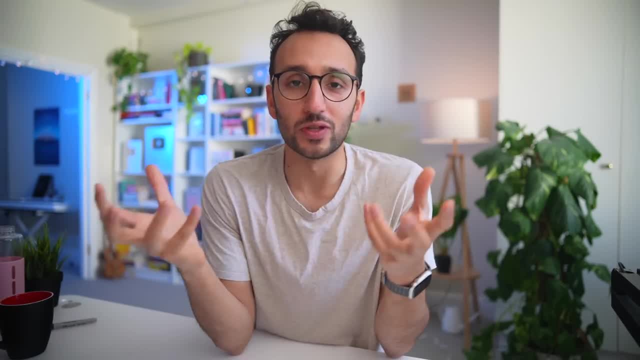 is Huel Black, which is often what I have in the mornings as part of my morning routine. It's 40 grams of protein, 400 calories. I just add water, blend it up in the Nutribullet blender thingy And then it turns into a genuinely tasty smoothie that has all of the right macros and all. 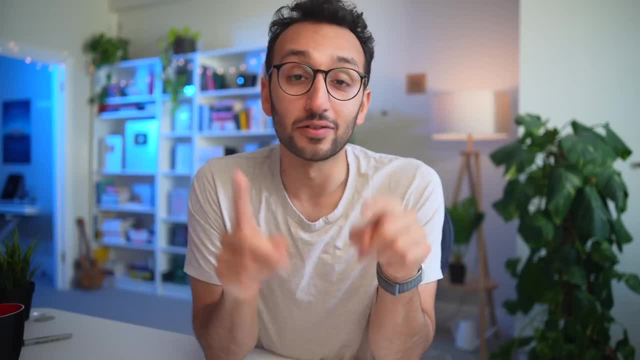 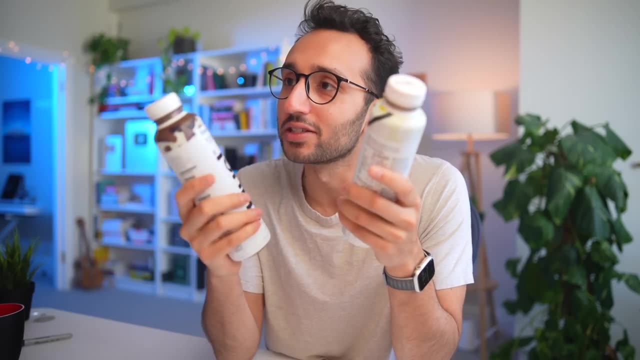 of the micronutrients that I might need for the day, And the other Huel product that I get a lot of value out of is the Huel Ready to Drink. And again, I've been getting deliveries of this ever since. I don't quite think this started in 2017, because this wasn't a thing in 2017.. I think like 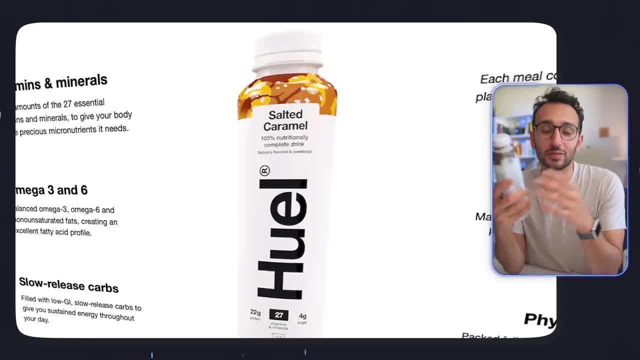 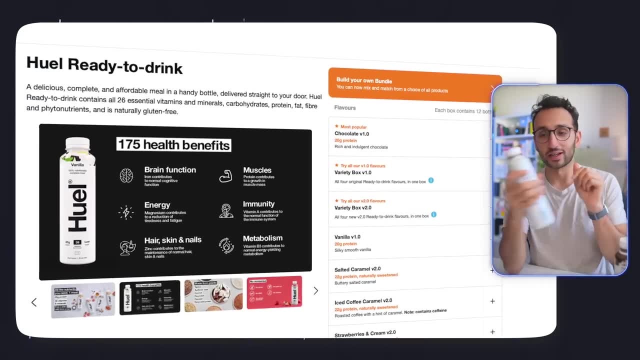 since 2020, this has been a thing and I've been getting regular deliveries of these And it's basically a whole meal that's 100% nutritionally complete in a single bottle, And if, on a given day, I don't have time to have a proper lunch, then the Huel Ready to Drink is an absolutely fantastic. lifesaver. My favorite flavor is banana. I think that's the best one, but all of the others are pretty tasty as well. Now, the best way of trying these, I'd say, is the variety pack, because it gives you like three bottles of all of the four different flavors, If you're interested in trying. 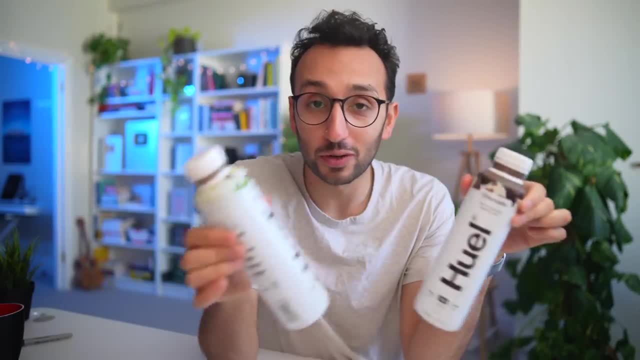 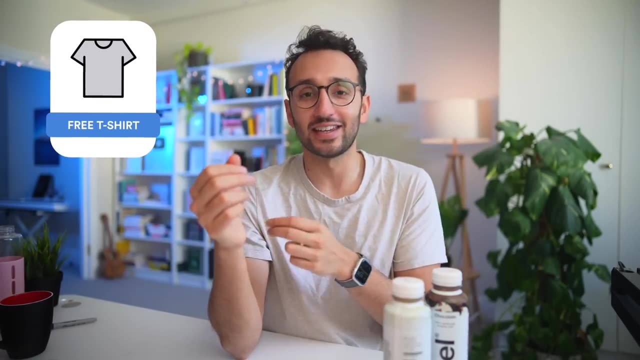 out any of these Huel products, including Huel Ready to Drink, then do hit the link in the video description And if you use that link, then you will get two free products along with your Huel order. You will get a free t-shirt, which is genuinely good and it's nice and elastic-y, and 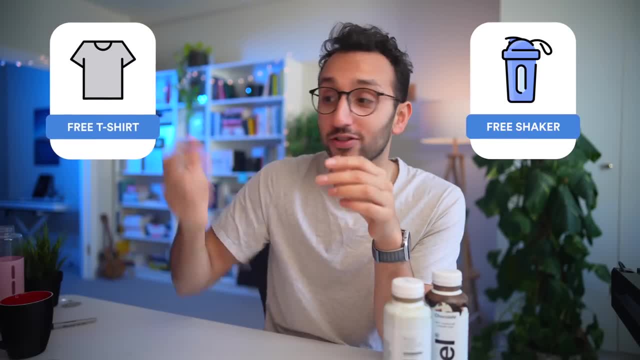 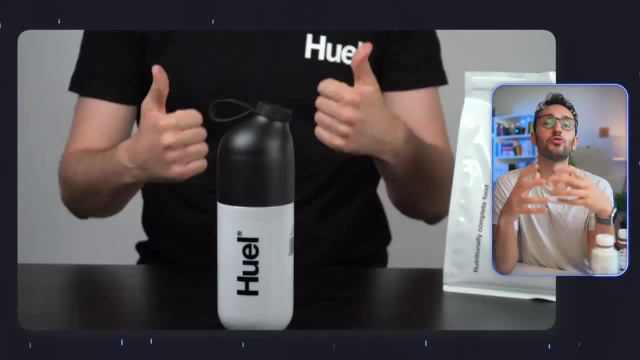 makes you look hench, which is a fantastic quality t-shirt. And you'll also get a shaker, so that if you don't want to use a NutriBullet blendery type thing, you can just put the thing, put the powder into the water into the shaker, shake it up and now you have a nutritionally 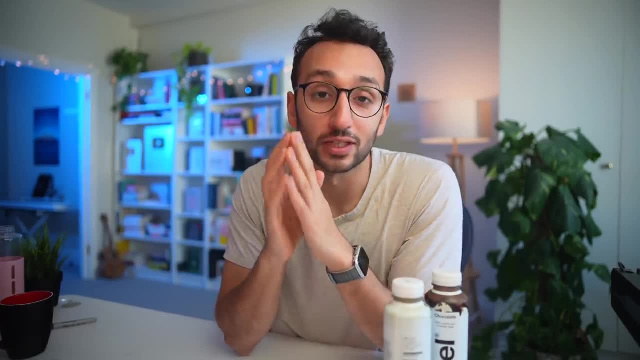 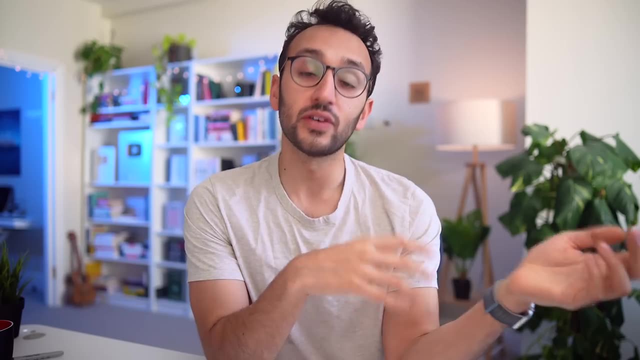 complete meal that's basically ready to go. So thank you so much, Huel, for sponsoring this video, And the point here is that basically, I want to define what are the containers of time where, in an absolutely ideal week- not necessarily a perfect week, but in an ideal ordinary week- 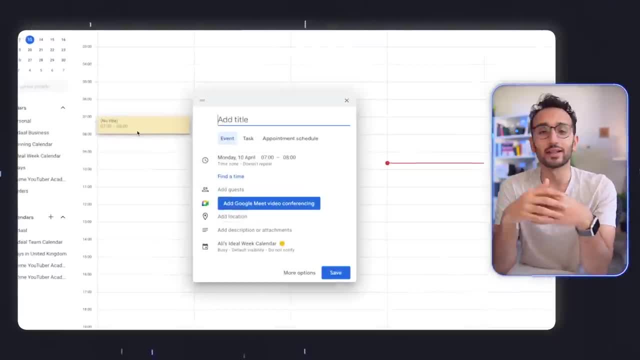 how would I choose to be spending my time? So, for example, I've decided that in my ideal week, Monday through to Friday, I'd like to wake up at seven o'clock and then I'd like to have the first hour of the day for my morning routine, And this is a thing that I've been doing for a long time. 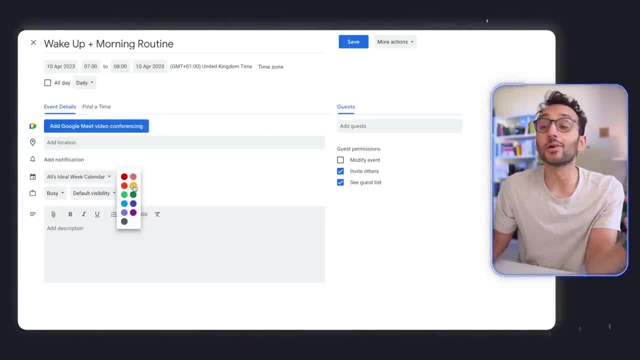 and this is a thing I'd like to happen every day, And so I'm going to repeat this daily and I'm going to give it this yellow color, because that like signifies the sunrise or something like that, And you know what. Why not add an emoji to it, just to make this a bit more? 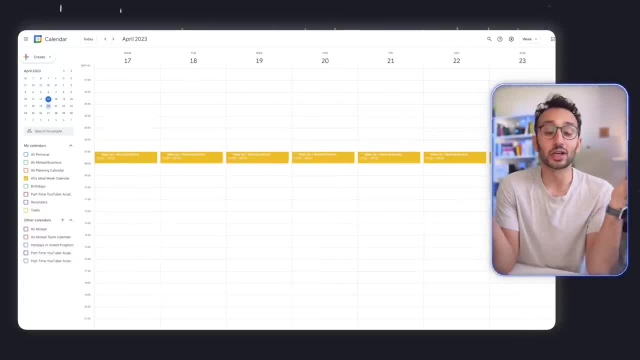 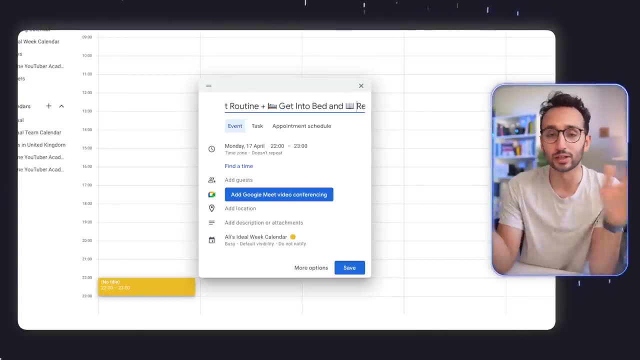 fun. So we can see that this has now shown up across my ideal week And because I want to get my eight hours of sleep, I want to aim to be asleep by 11 PM And therefore I want to be starting to get ready for bed around 10, doing my reading nighttime routine. all that fun stuff. 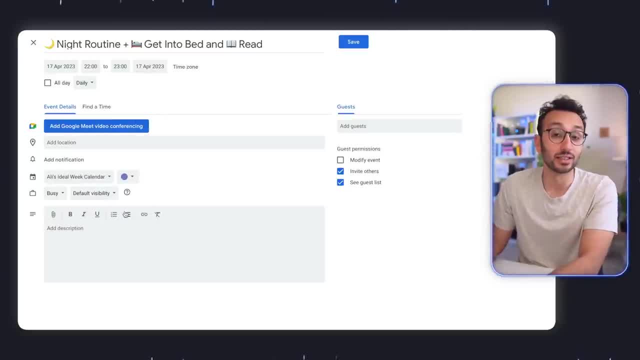 And I'm going to repeat this every single day, And I'm going to give this a lavender color to signify nighttime- Fantastic. So we now have a block for waking up and we have a block for sleeping, And now I can figure out what I want my ideal ordinary week to 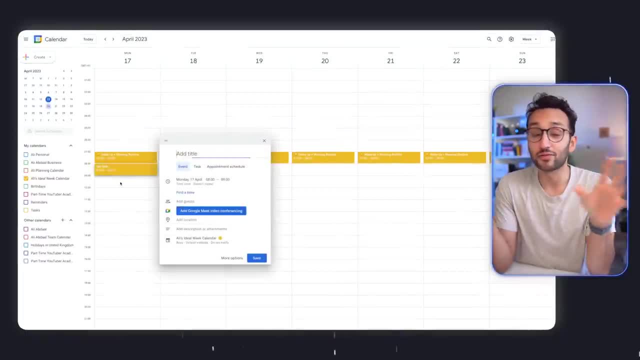 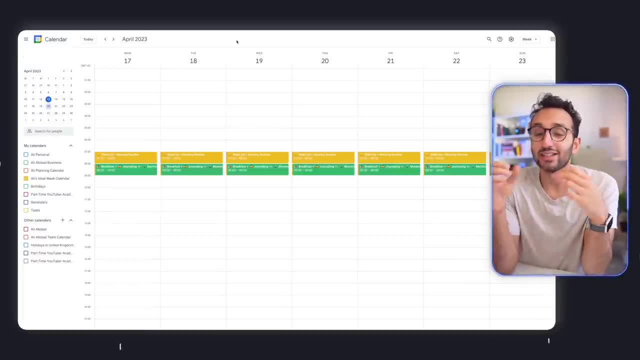 look like in the rest of the time. I've decided that in my dream world, from eight till nine every morning I'd like to do breakfast and journaling, And in that block I could maybe have a breakfast meeting with someone or maybe go for a walk. And then I want my actual quote work day to start at. 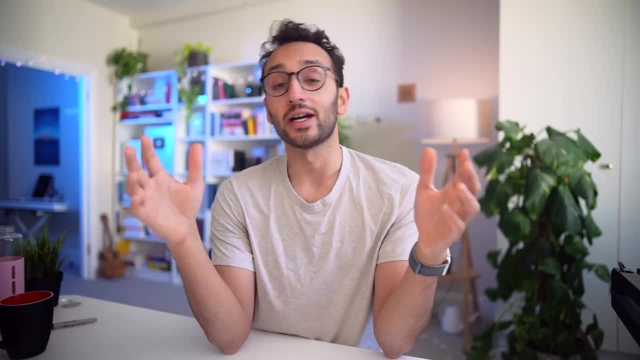 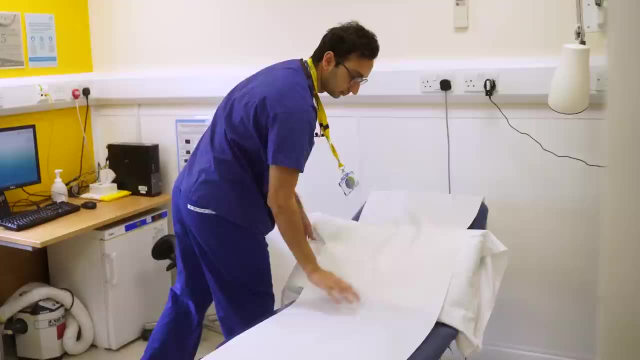 9 AM every day, And so, based on my own energy levels, how would I like my ideal work day to go? Now, obviously, this is going to vary a bit depending on how much control you have over your own schedule. For example, when I worked as a doctor, I just had my entire block being. 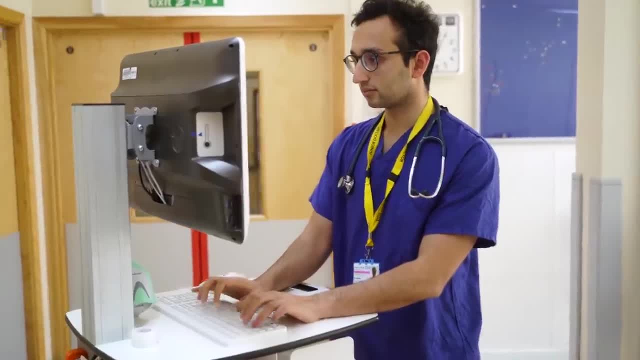 like nine to five work day or whatever this shift was, And then I would just have to do whatever just happened on the day. I couldn't quite decide, you know what. These are the things that I'm going to do. I'm going to do this, I'm going to do this. 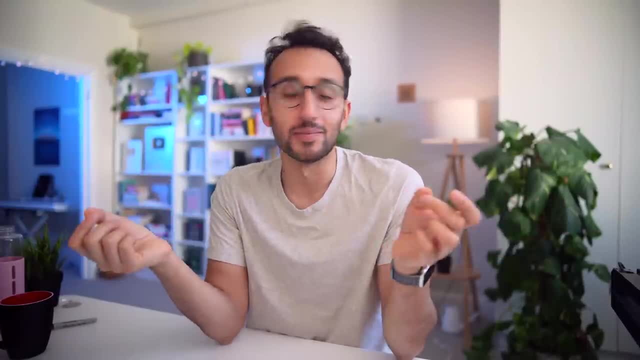 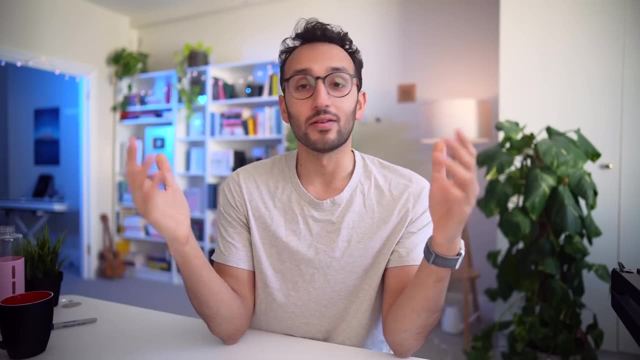 These are my four hours of deep work time, But as an entrepreneur, I can decide how I spend my time, And actually increasingly in jobs, especially in knowledge work, you actually do have the ability to talk to your boss or your manager and say, hey, this is how I work best. I would love it if we can. 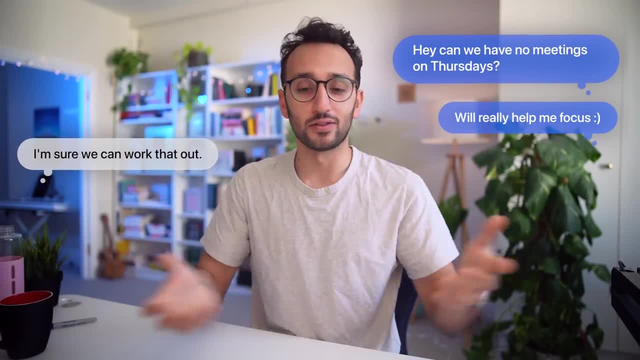 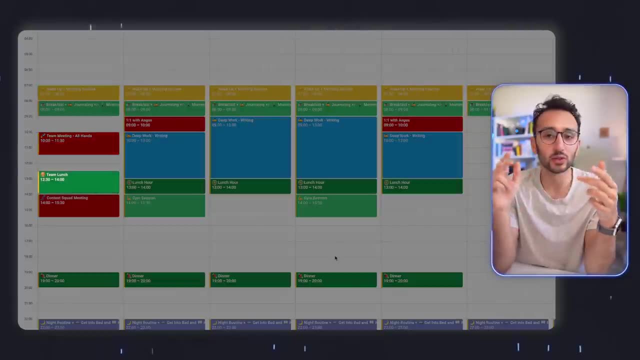 find a way to fit my calendar around this And then, obviously, based on the needs of the business and the team or whatever things, will have to adjust accordingly, And so I've added in the blocks for the weekly team meeting. weekly team lunch. weekly content squad meeting. 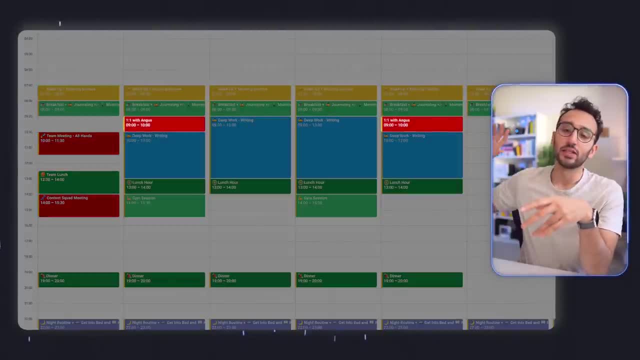 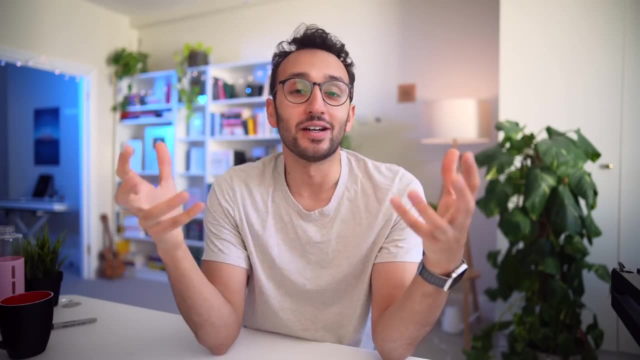 and my two meetings a week with Angus, who's my general manager, And I've added in the blocks for when I want to have lunch roughly and the blocks for when I want to have dinner on weekdays, And this is already very helpful, because now I can see what is the other time that I have to play with, And then I can adapt this. 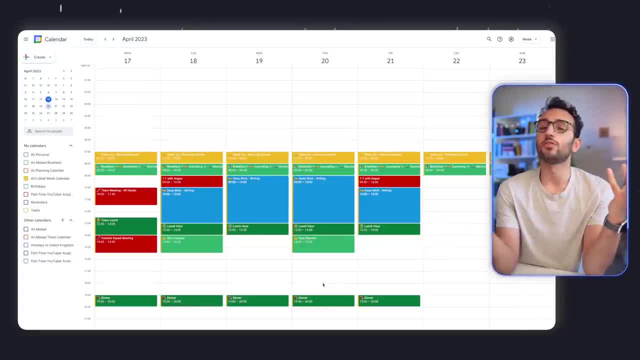 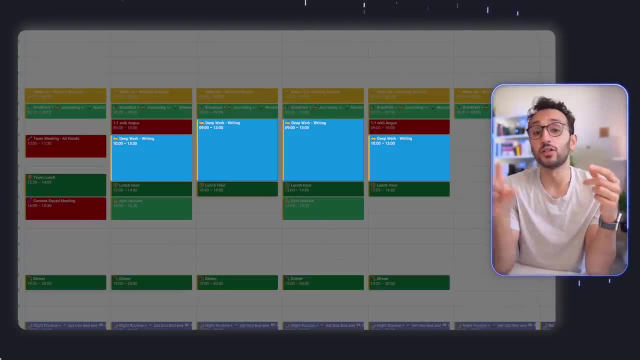 ideal ordinary week based on how I'd actually want to spend that time, And so Tuesdays to Fridays, for example, I want to have several hours in the morning as a deep work block for writing, And in my ideal week I'd like to do a gym session Tuesday afternoon, Thursday afternoon. 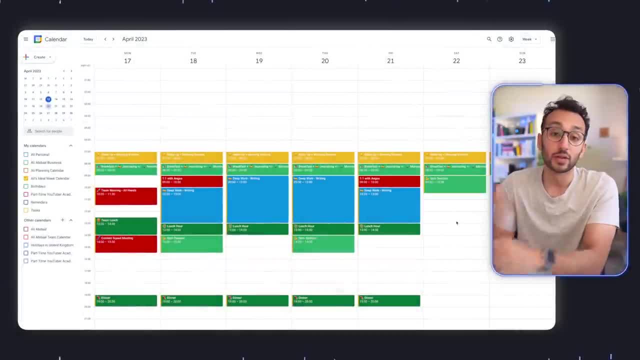 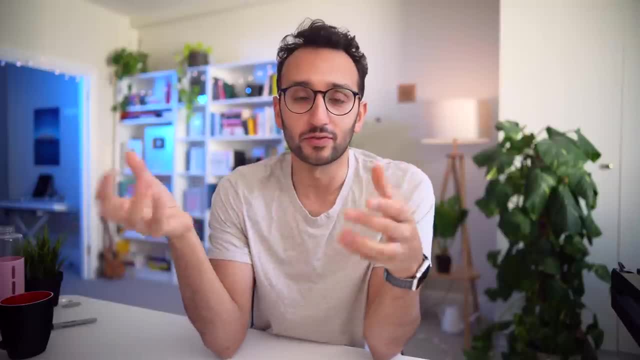 and maybe Saturday morning, if I happen to be free on the Saturday morning. Now the other main thing I need to do in my workday is filming, And so I'm going to put in my various filming blocks into the calendar, And obviously this workday schedule is very specific for me. 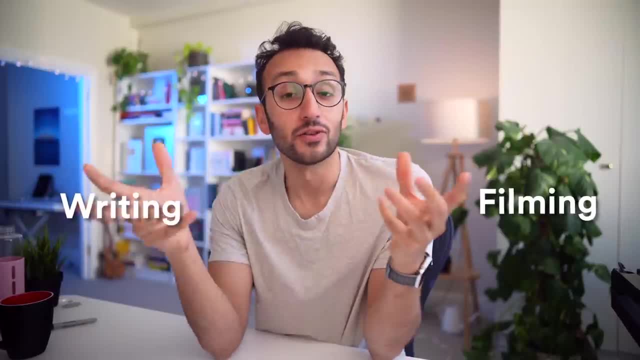 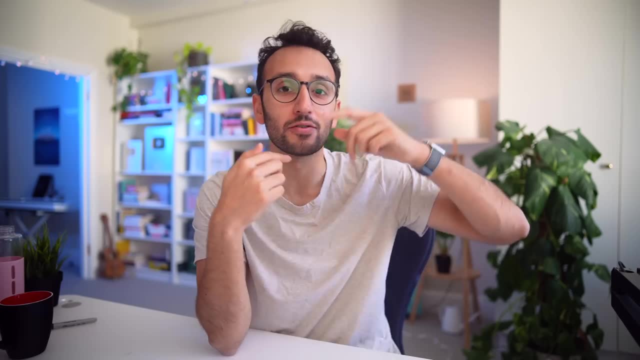 because basically all I have to do in my job is writing and filming. But if your job is a little bit different than that, then maybe you might have a block for checking Slack or checking emails And you might do that once or twice a day so that you're batching those interruptible activities. 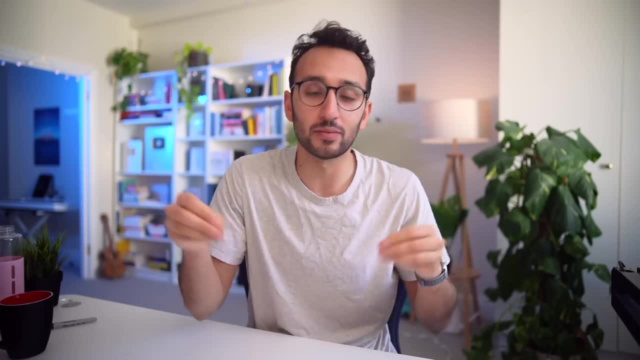 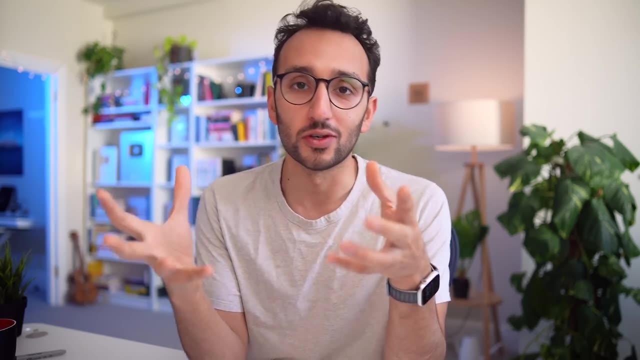 and you're not just spending your entire day being derailed by all the various emails coming your way. Alternatively, maybe you have more meetings than I do and therefore you have more meetings in the calendar at all the different blocks. The point is, mold this to whatever works for you, But the 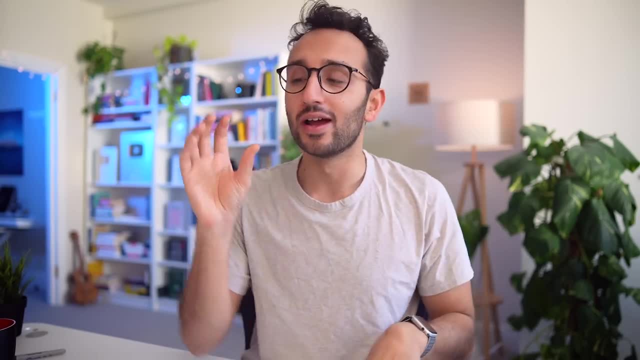 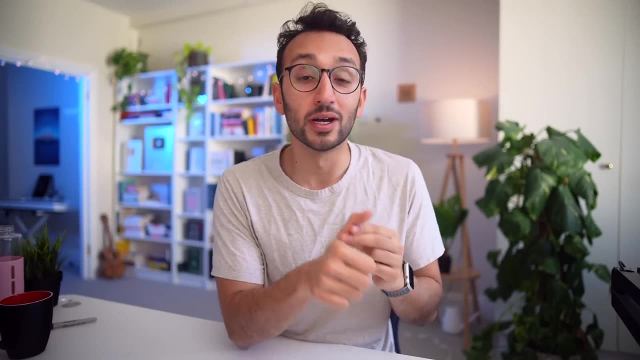 point is, we want to create these containers within our ideal week, where, in an ideal ordinary week, we would be intentionally using our time. and this way, And what you can base these containers on is, firstly, what are the constraints of your job, But also, how are your own energy levels Like? if you're managing your own energy, do you do your? 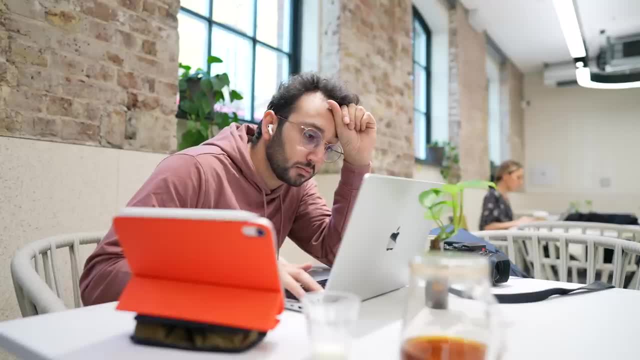 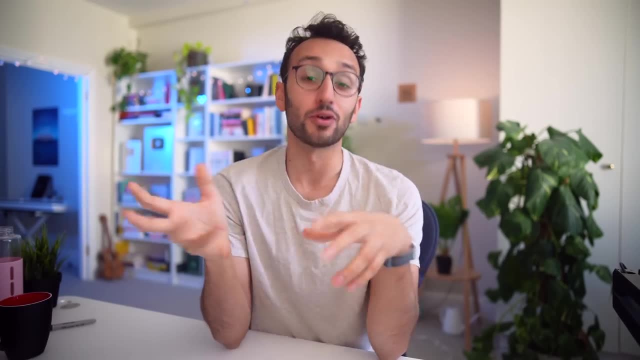 best creative work in the morning or in the evening? Do you have a slump after lunch And therefore maybe you want to take calls then rather than do particularly deep work? And the great thing about this and what I do is that I also intentionally schedule in the personal life and 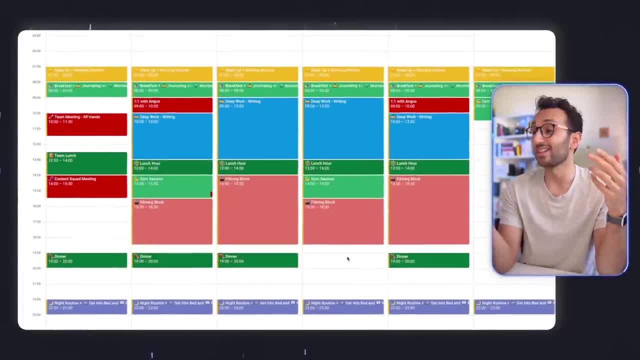 relationship, stuff that I want to put into my ideal week. So, for example, in my case, ideally every Thursday evening is date night, So I know that I have that fully scheduled in the calendar and now the rest of my life can fit around that. 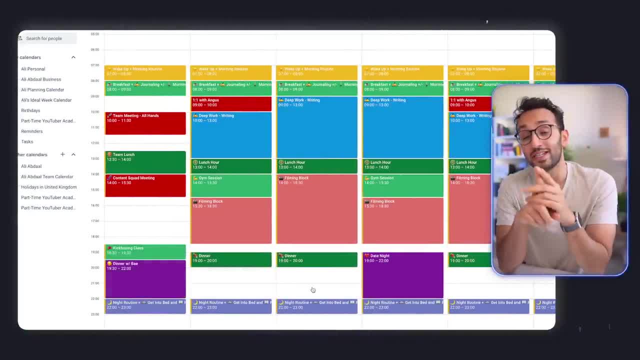 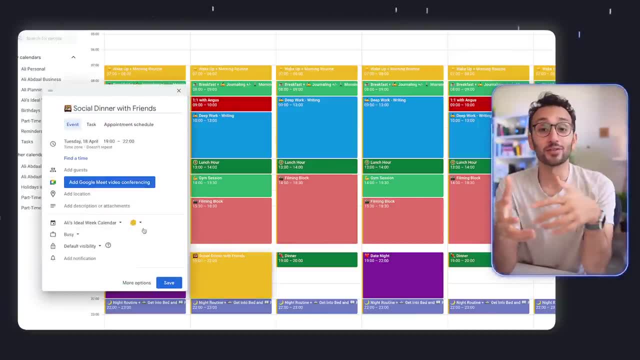 And then, on Monday evenings as well, I'd like to go to a kickboxing class and have a mini date night as well. In my ideal week, Tuesday evenings would, for example, be a social dinner with friends, because I'm trying to learn how to cook and I like having friends over, And so I've decided to just 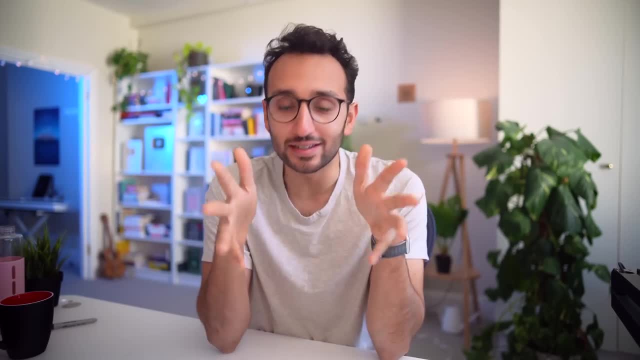 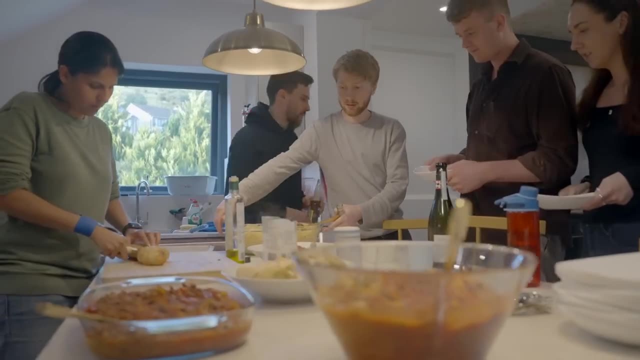 by default, every Tuesday evening is going to be free, so that I've got an easy slot where, if a friend is visiting London or if I want to invite people over, just by default, I don't have to think too hard about it. It's a Tuesday evening and, conveniently, the cleaner rocks up on a 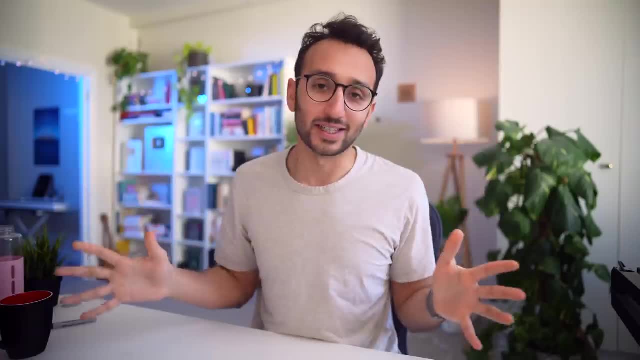 Wednesday, And so I can leave the kitchen in a mess and then the cleaner will sort it out. That's fantastic stuff. I might decide on Wednesday evenings- by default I'd like to drive to the drive home to have dinner with my mom and grandma, And I might decide to leave weekends. 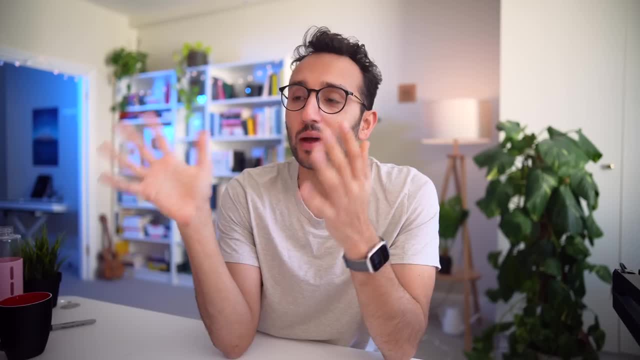 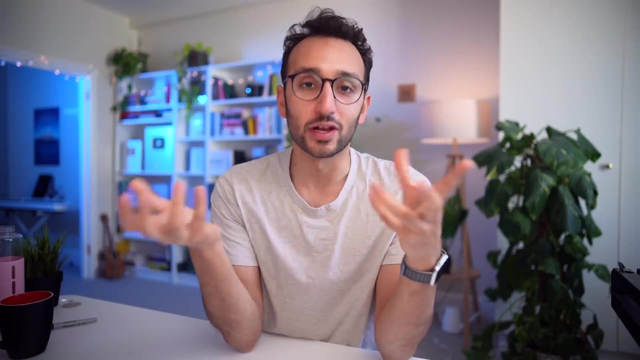 completely free for friends and family and other things in life that are happening Now. having this laid out in front of me is incredibly useful, And this is, in fact, the system that I follow basically every week, And then obviously there's other stuff that kind of derails this sometimes. 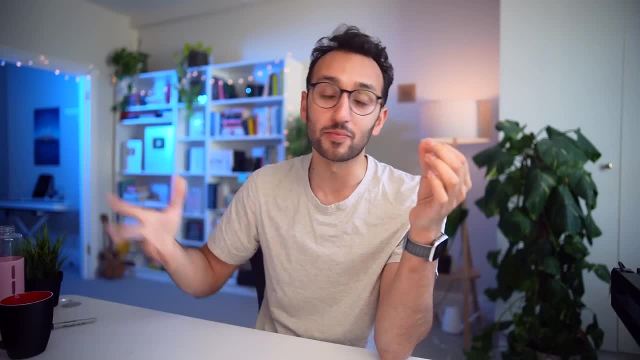 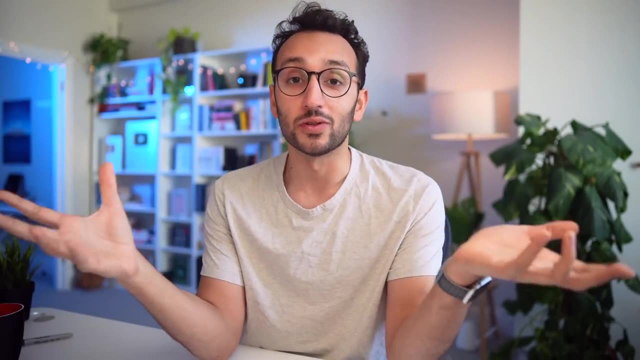 Sometimes there's an urgent meeting that can't be missed, or sometimes I have to go pick up my mom from the airport and then a filming block gets derailed. But the point is I have defined the parameters of my ideal ordinary week, And now I don't need to be fully wedded to them. 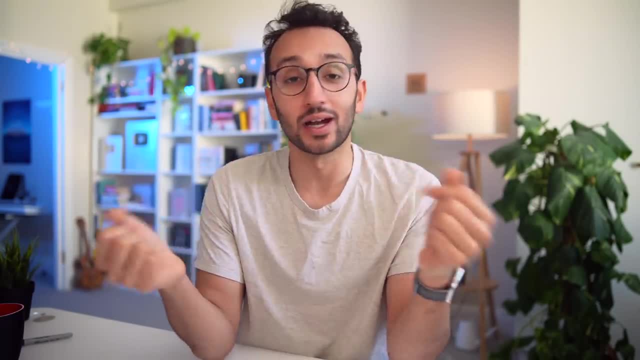 but at least I've actively decided that, on average, on a Wednesday morning, I'd like to be doing a deep work block every single day. So I'm going to be doing a deep work block every single day, Writing, because that's the main thing that moves my business forward And it makes sense to do that. 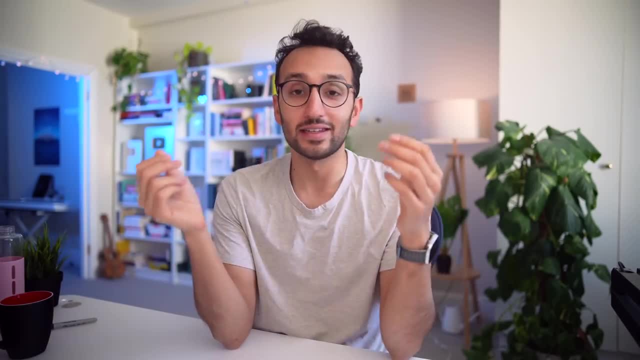 in the morning, while I have more creative energy. Similarly, the fact that I've basically decided that Mondays and Thursdays are going to be date night, that that means that those evenings are sacred, And like if someone says, Hey, do you want to hang out? And it's Monday or Thursday night. 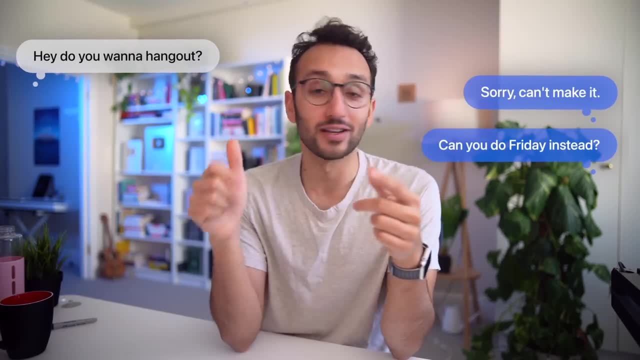 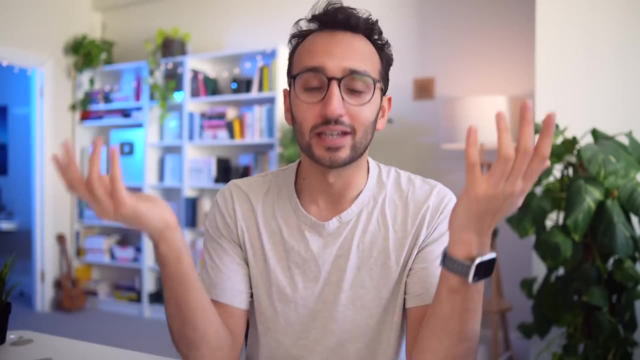 then my default option is: no, sorry, I can't make it. Can you do Tuesday instead, or Friday instead? And if it's super, super urgent and it's like an internet friend visiting London and they're only here on a Monday, then I can say to my girlfriend: Hey, do you mind if we switch date night to 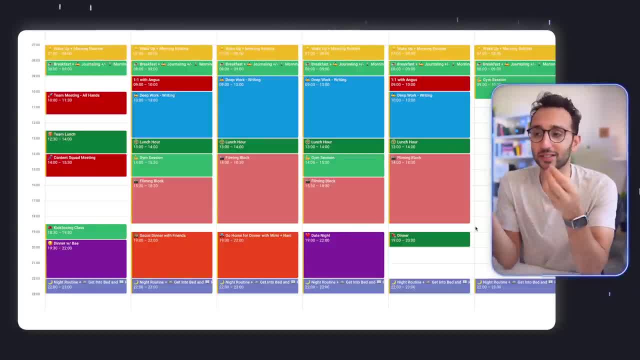 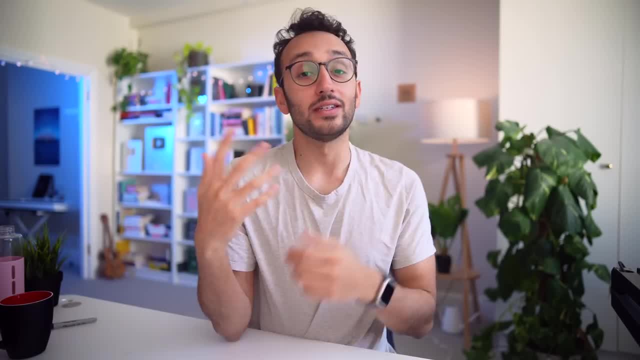 Tuesday or whatever that week. So the point is, this kind of system allows a level of flexibility And I've found that over the last eight months of using it it's just freed up so much headspace from my life having to think about these things, because now at least I have a default structure. 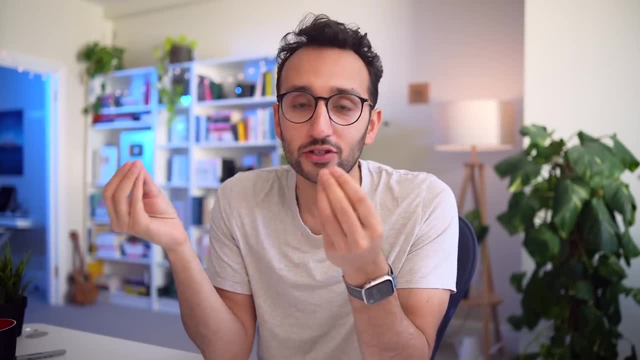 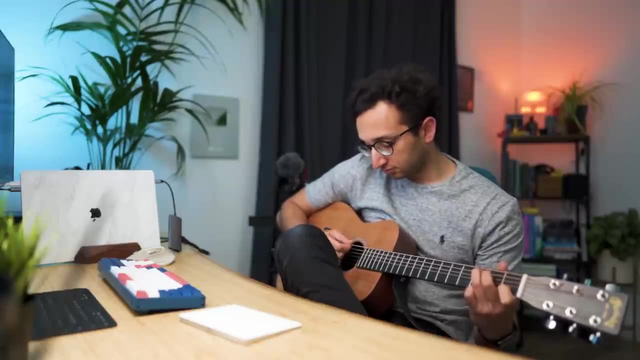 that I can follow. The other cool thing about this is that it really shows where- genuinely where- is the free time, Like I might decide. you know what I'm really interested in? the guitar. I want to get better at the guitar And therefore I'd like to have one guitar lesson every week. 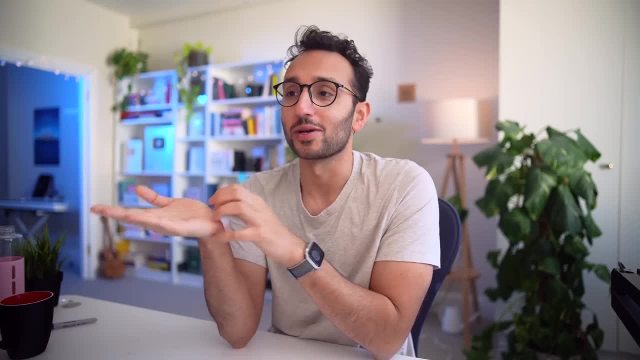 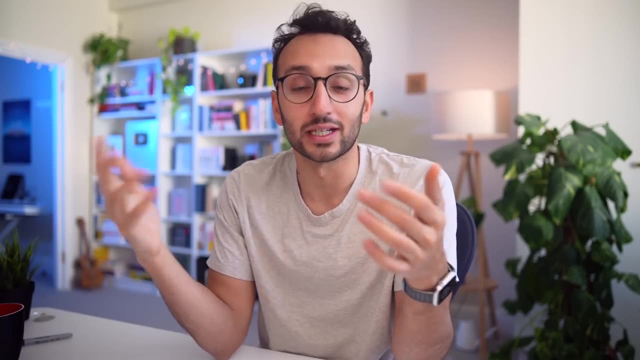 Now the question is: where am I going to? where am I going to fit this one guitar lesson every week? I have these 112 hours that I can play with, like everyone else does, And so I might decide. you know what. I'm going to finish work a little bit earlier on a Wednesday to have my guitar. 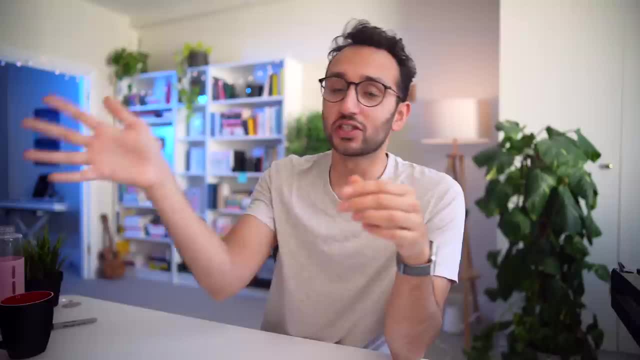 lesson. I'm going to finish work a little bit earlier on a Wednesday to have my guitar lesson, But I can do that because I'm an entrepreneur and I control my own time. But if this is what my calendar looked like- and I was only getting home from my actual job at like 6: 30 every day- 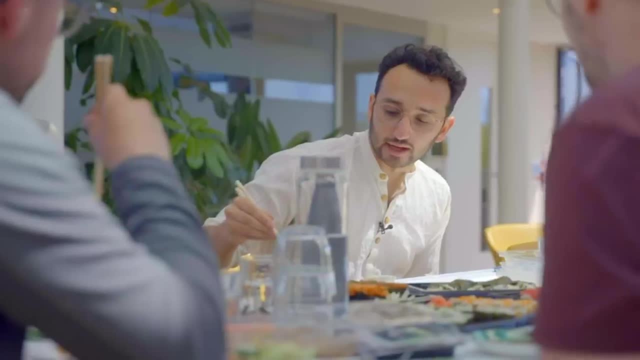 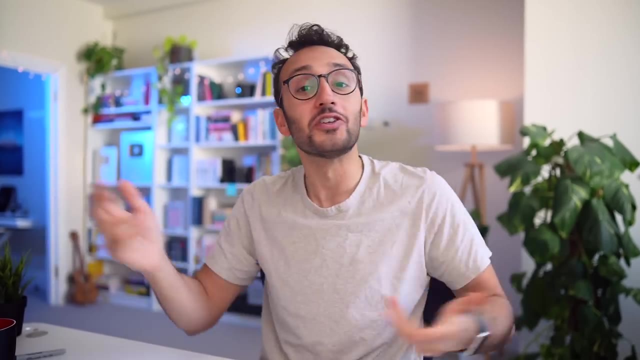 and I knew that I wanted to have a social evening with friends once a week, go home for dinner with my parents once a week and have date night twice a week. It's like I actually don't have that much time to play with to fit in a guitar lesson, And that means I don't need to beat myself up. 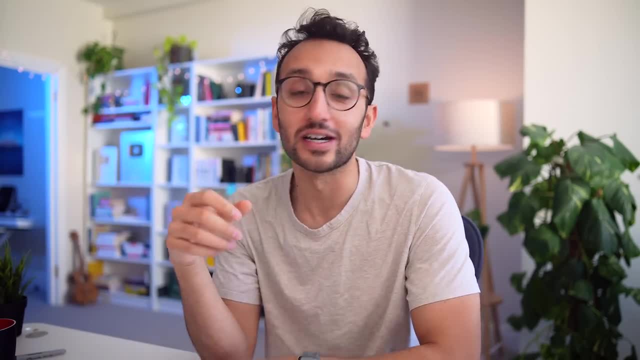 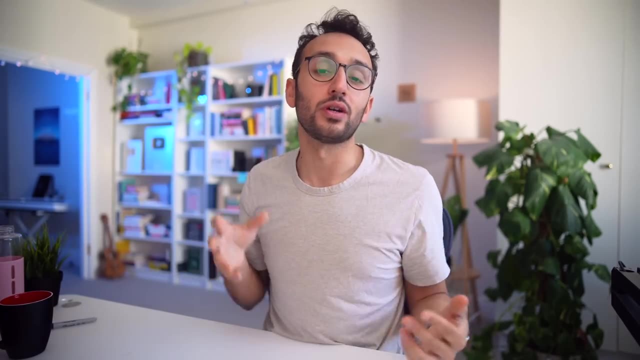 about it. I might think you know what, At some point in my life, when I have more free time on the calendar, I will fit in that guitar lesson, but it's just not a priority right now. And what I love about this Ideal Ordinary Week exercise is that it forces us to decide what are the priorities. 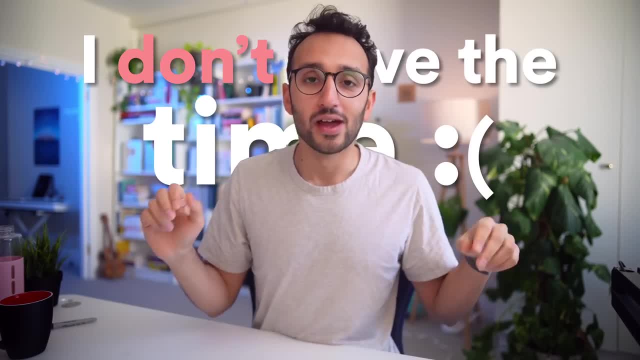 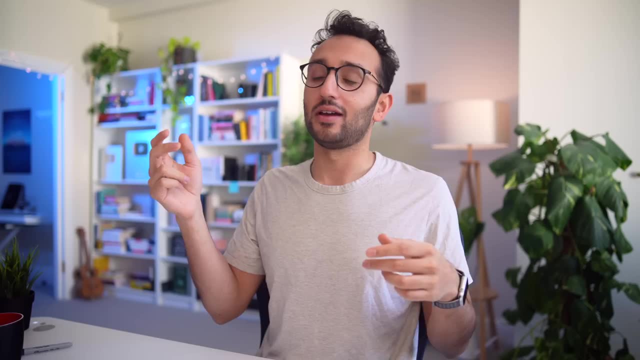 in our life. It means we can't say, oh, I don't have the time. We can instead say I'm choosing not to make the time. I'm currently choosing not to make the time in my life for guitar lessons or singing lessons, And I'm currently choosing in my life to only go to the gym two or three times a. 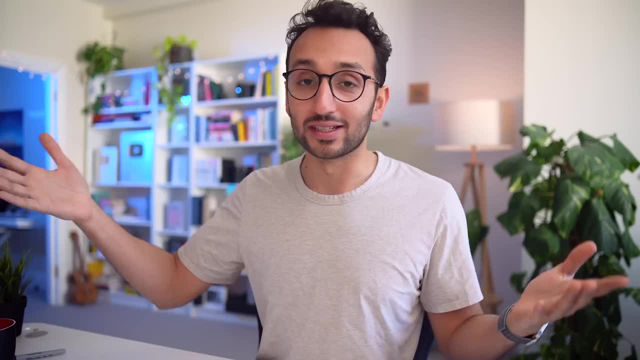 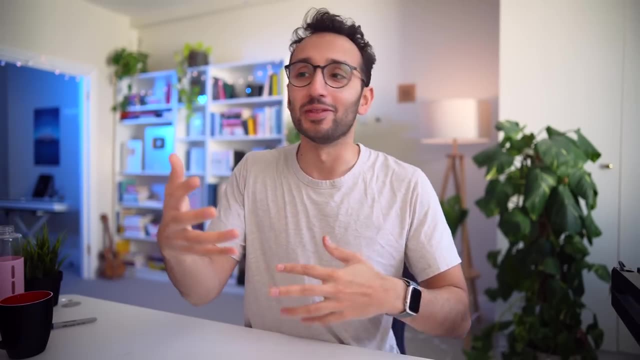 week, because I've decided that that's what the priority is In the future. maybe once my book is done and I have fewer writing blocks, or maybe I decide- you know what, I want- to take a break from filming four times a week for a month and see what happens, I'll free up more time. But the point is: 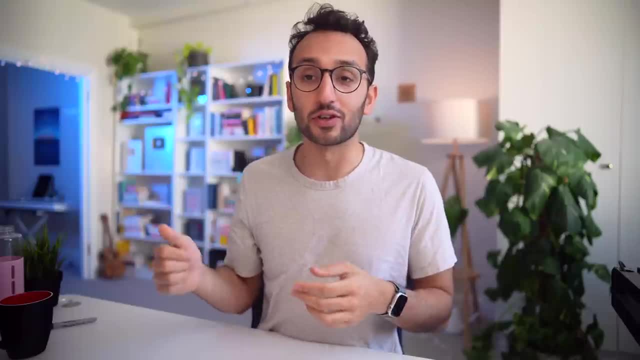 I now know how much time I have to play with, But until I did this exercise eight months ago: A I would not have known that And I was kind of taking on too many responsibilities and too much stuff and then feeling overwhelmed And B. 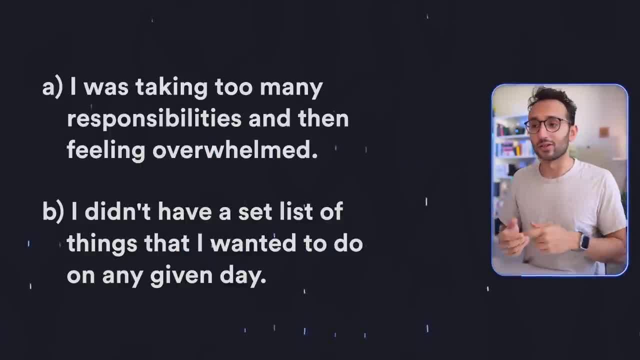 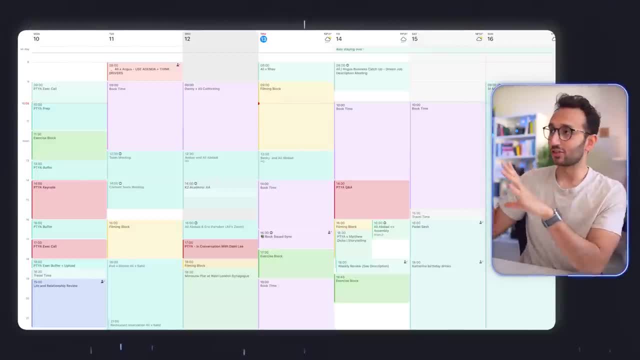 on a given day, I didn't really have a default list of things that I wanted to do, And so I'd have to think every single day. I was like, okay, how do I want to spend my time today? And that's just quite a lot of thinking. Now, this is how this actually translates to what 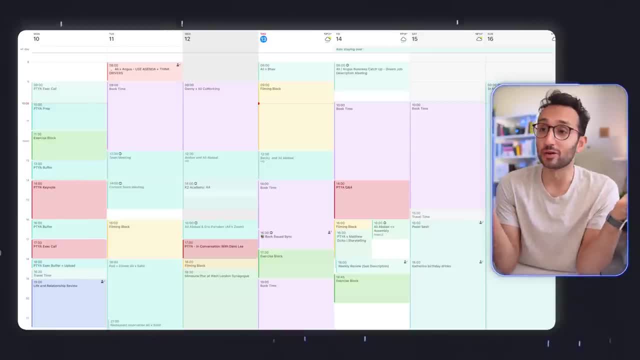 my Ideal Week looks like in real life. So right now we're in the midst of our Part-Time YouTuber Academy, So Mondays are literally taken up entirely with PTYA stuff, except an exercise block in the morning, Tuesday morning, Wednesday morning, Friday morning, Saturday morning. 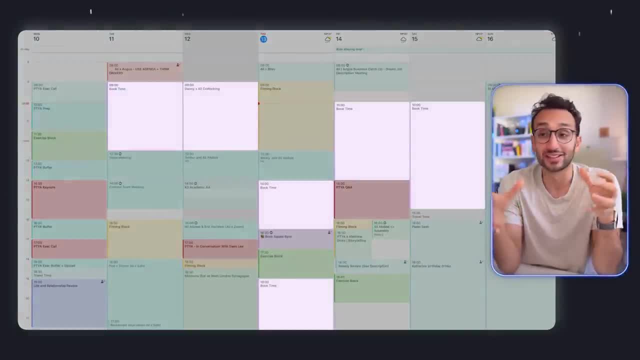 and Thursday afternoons are all book time because I'm in the final stages of my book And so I need to make the blocks for that. I have various meetings in the calendar, So we've moved our team meetings to Tuesday. So we've got our team meeting and our content meeting on a Tuesday. 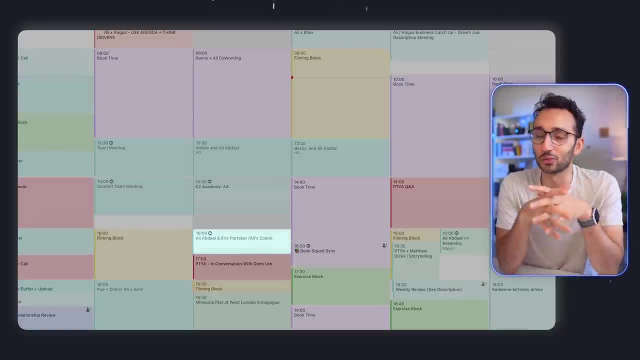 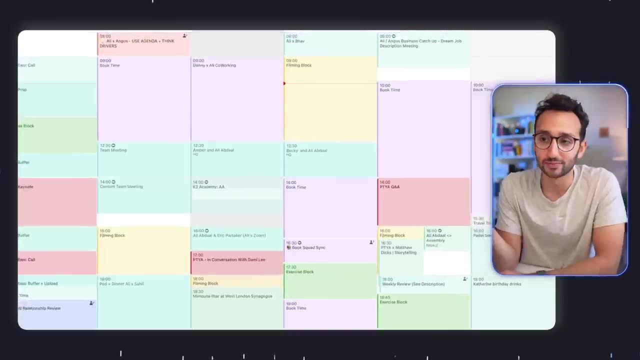 afternoon We're doing a team training thing with our coach, Eric, And so that happens on Wednesday afternoon, And this week I've had various lunches with various team members, because I like to have a one-on-one lunch with every member of the team once every couple of months or so. Similarly, 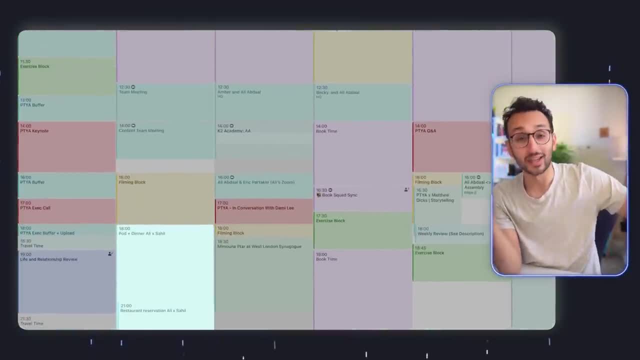 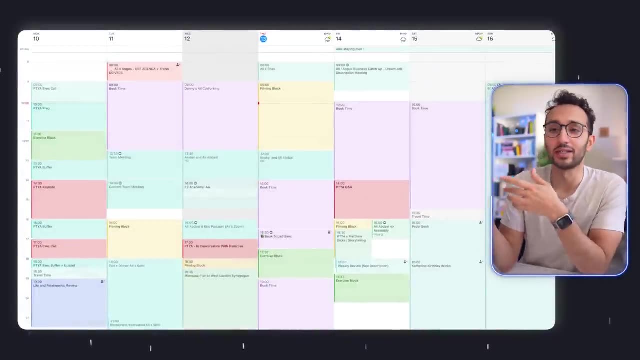 this week I did a podcast with my internet friend, Sahil Bloom, So that happened on a Tuesday and then we went out to a restaurant. So you can kind of see how this calendar evolves over time. and it evolves depending on what's happening in a given week. But this week I've brought 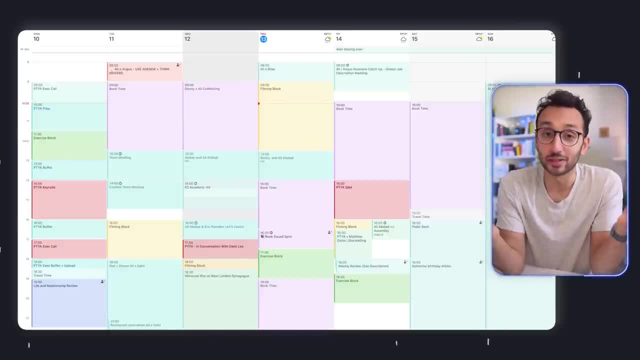 really stuck to the calendar. I've done book time when I intended to. Currently I'm in a filming block, which is why I'm filming this video, And then later today I've got book time for the rest of the afternoon, so I can focus on making those final edits And it's just so. 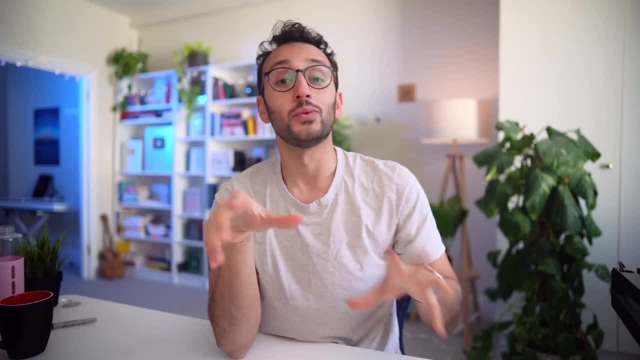 liberating to have this kind of system. I'll put the template for the Google Calendar Ideal Week, if you want to check it out, down in the video description. Again, it's completely free. You just click the link and you can download the template. And if you try, any of the strategies, 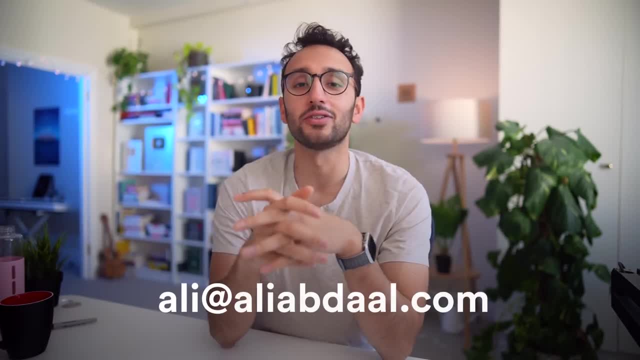 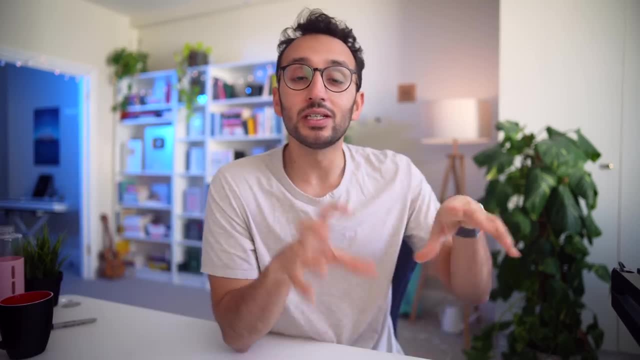 in this video. I'd love to hear how you got on. Please can you drop me an email, alialiabdaalcom. I read absolutely everything, even if I can't reply to everything, And I'd just love to hear kind of what are the strategies and tips you found helpful, And maybe you can even leave a 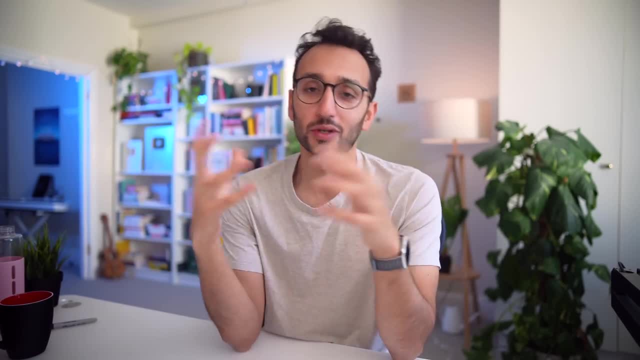 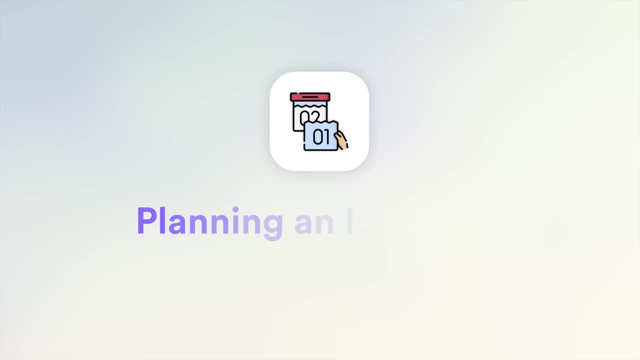 comment down below. if you try any of this stuff out Again, I'd love to hear what are the pros, what are the cons, what are the ways you've adapted it to fit your own system and your own life. All right, the final component of the Trident Method is what we do on a given day. 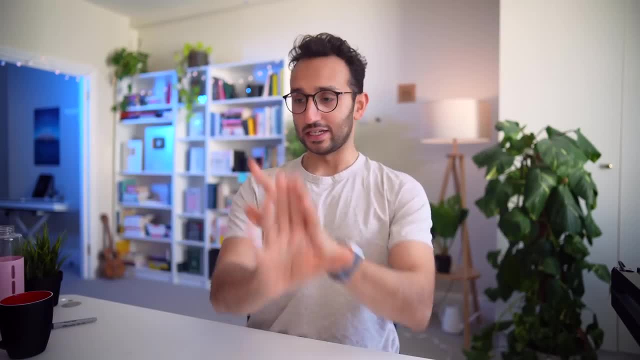 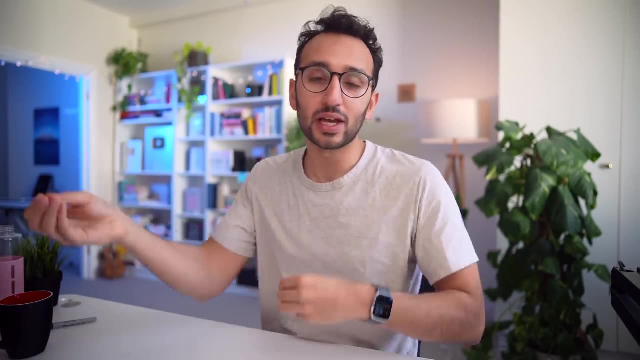 So we've talked about annual planning and what our annual life plan Euro at a glance looks like, And we've talked about, at the level of the Ideal Week, how we're trying to make the most of these 112 hours in the week that we have to play with, and 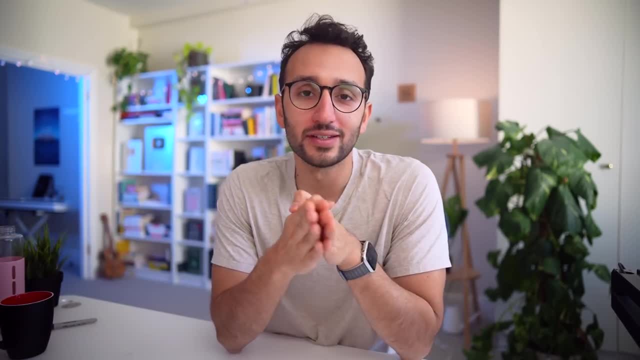 how we can use them more intentionally. And so now the third component of the Trident Method is what we're doing on a given day, And so the way I manage my time on a given day is, broadly, I follow what is in the Trident Method, And so the way I manage my time on a given day is, broadly, I follow what is. 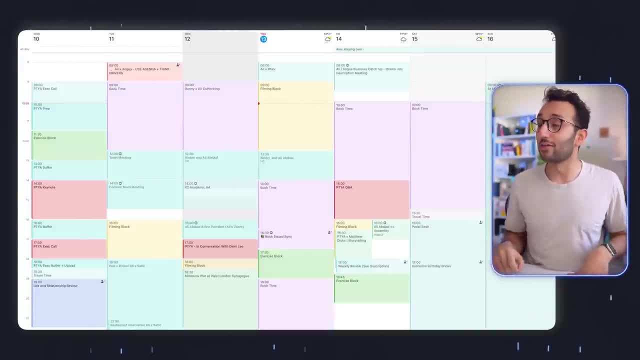 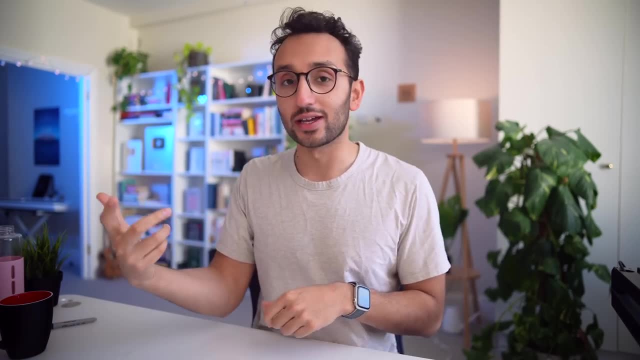 in the calendar And again, having the calendar just makes it so easy. It is a Thursday right now and I just literally follow whatever blocks I've put in my calendar And generally on the weekend before I will look forward at my calendar for the upcoming week and I will create blocks of time for 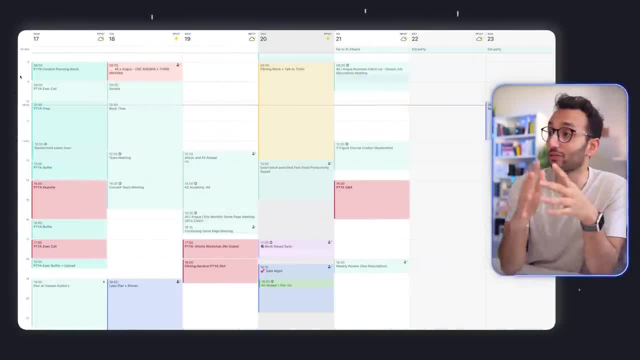 the things that I want to do, And so, for example, let's say I'm looking over to next week. I've already got a lot of this stuff penciled in because it's recurring events or it's Ideal Week stuff And because I know that basically every morning I want to do book stuff and every afternoon I want 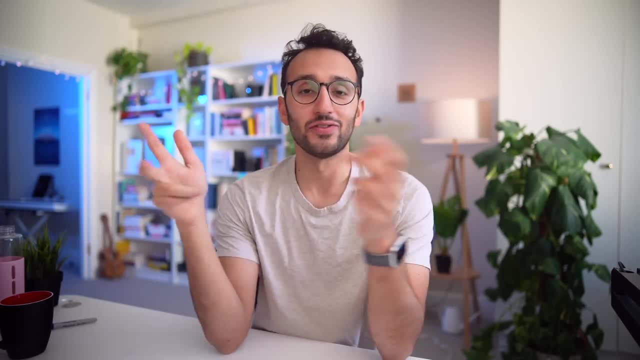 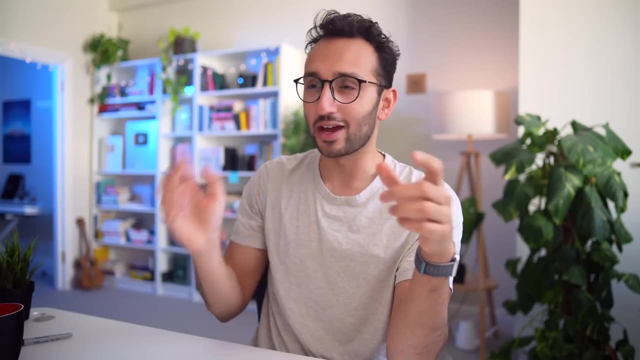 to do kind of filming stuff and I want to go to the gym two or three times. I just need to add in those blocks, And normally I'd have those in as like repeated blocks. that's just in every week. but right now things are very derailed thanks to the YouTuber Academy, And so I'm kind of going. 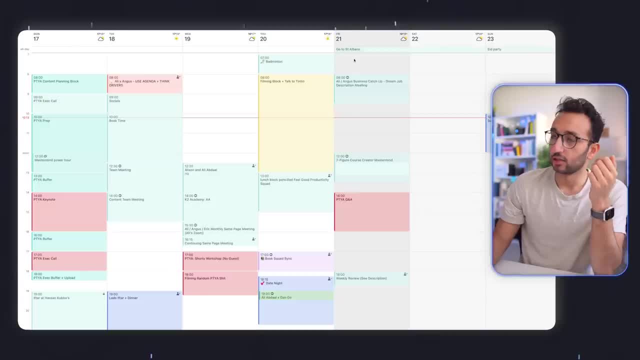 week by week, But keeping in mind what does my Ideal Week actually look like? So, for example, right now 7am badminton is not happening, So let's decline this one. Let's create a book time block on Wednesday morning. Let's create a book time block on Friday morning. This app is Fantastical. 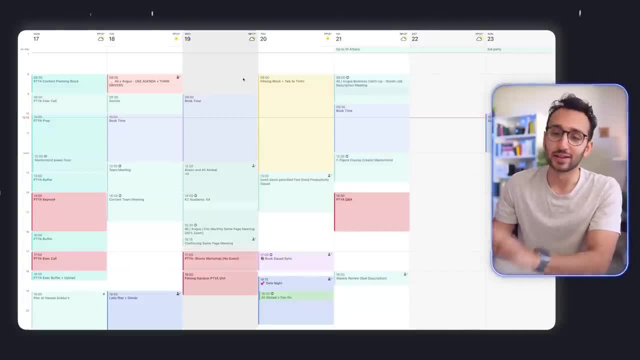 by the way, it's just a fancy calendar version of Google Calendar. The nice thing is you can duplicate events, So it makes it super easy to like literally hit alt and then drag, and now I can just duplicate an event, Rather than having to recreate it like I would in Google Calendar. Let's put in my filming blocks. 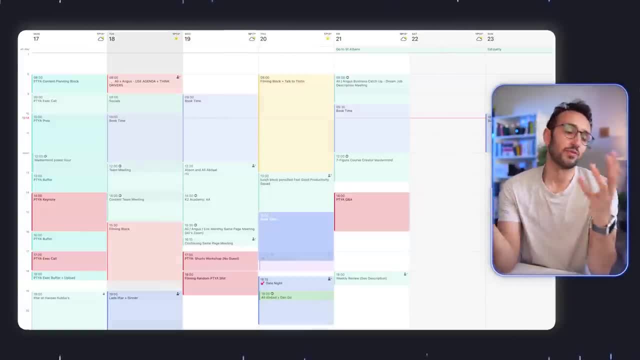 Now this is currently a bit of a problem because I don't have enough time for exercise here, So I'm going to have to create some exercise blocks. But then genuinely on the level of day planning- let's say it was Monday- I would literally just follow whatever I have planned. So I know. 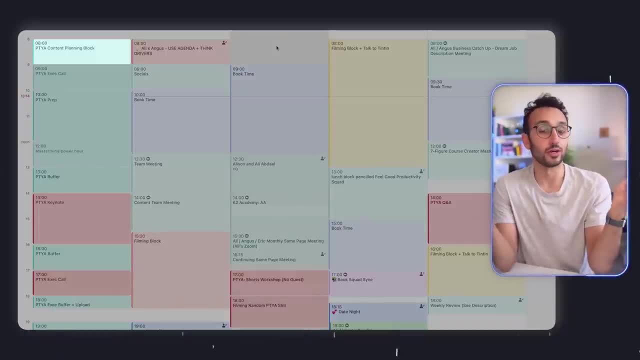 for example, at eight o'clock I'm going to be doing my content planning for the session of the Part-Time YouTuber Academy. I've got my call with the exec students at nine and then another one at five. I've got more PTYA prep happening from 10 to 12.. I have a YouTuber's 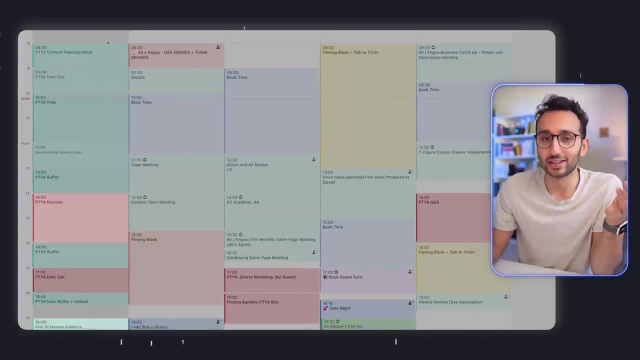 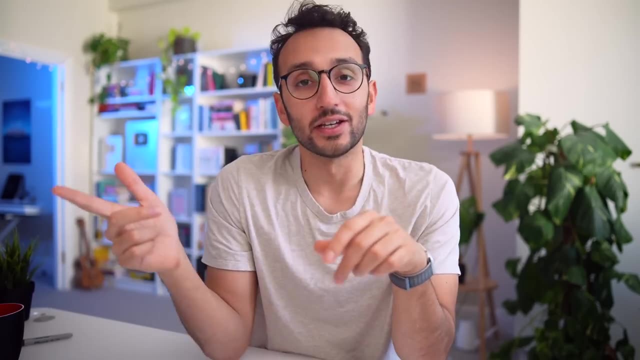 mastermind that I'm part of, I have the two hour keynote that I deliver on a Monday, And then I'm going for aftar and dinner at a friend's house that evening, And so on one level, that's just what I do on a given day. I just follow whatever's in the calendar. But there's another thing that I 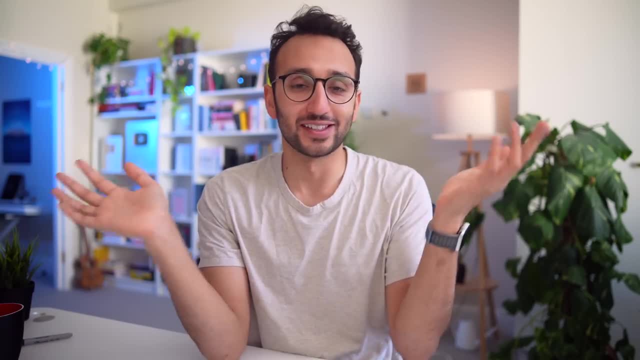 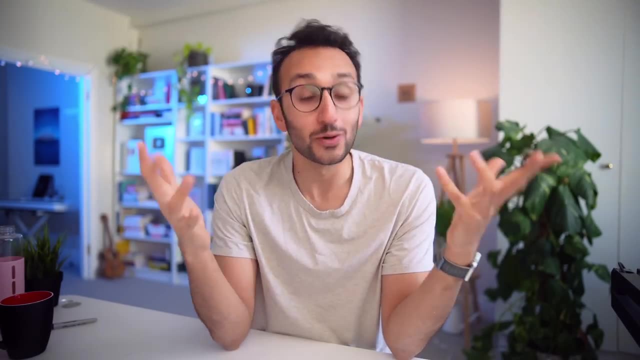 do And again, this is one of those things that I've started doing for the last eight months, ever since starting working with Eric, And it's basically defining three daily quests. Daily quests, I mean, he calls it daily number ones or whatever. I call it daily quests because 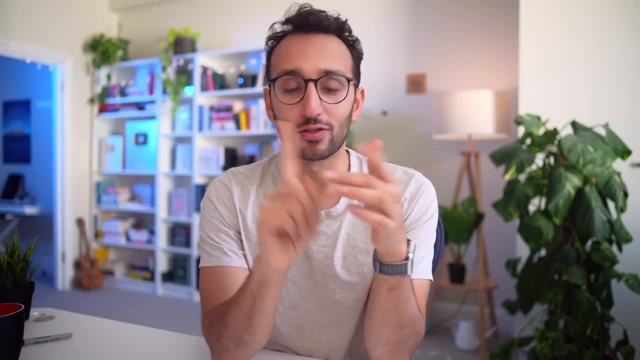 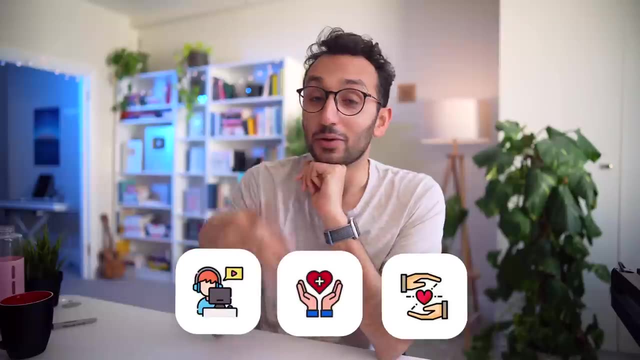 it's terminology from World of Warcraft, And basically the idea is that in the three most important domains of life, I have three quests that I'm doing every day, And that's in work, in health and in relationships, And we've actually recently started a Slack group. 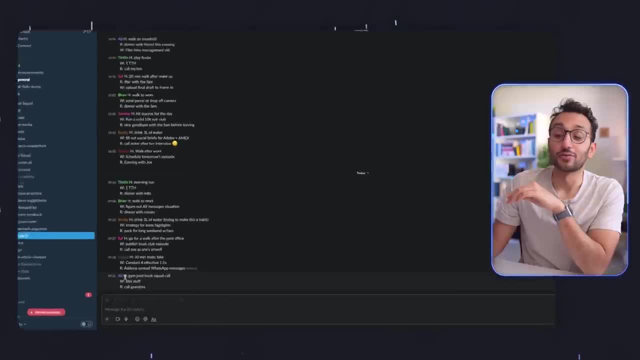 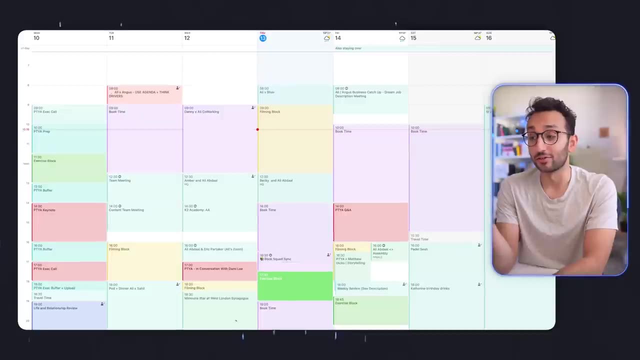 we do this with the whole team so that we've got some level of accountability on this. And so, for example, today my health daily quest is to go to the gym after my book squad call, and then I make sure it's scheduled in the calendar So I already have my exercise. 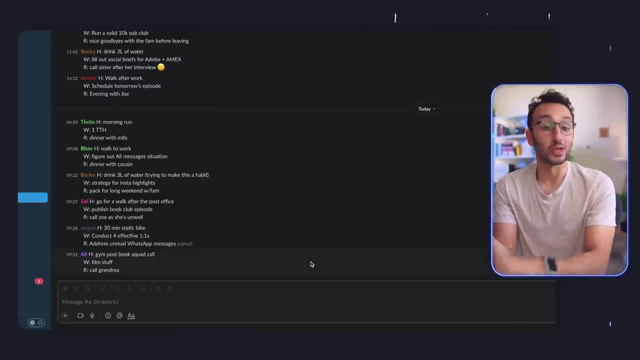 block scheduled in the calendar after my call with the book team. My work daily quest is: I want to film stuff which is literally what I'm doing right now And that's already in the calendar. And then my relationship thing is that I want to call my grandma. 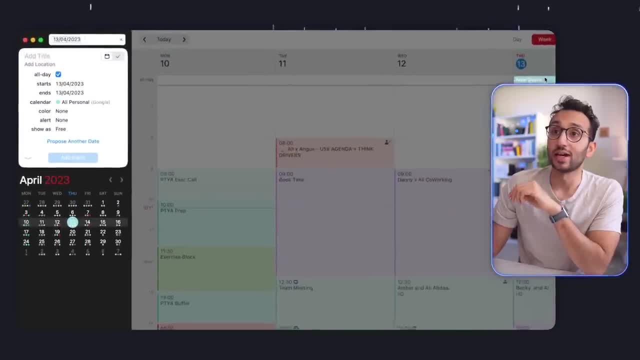 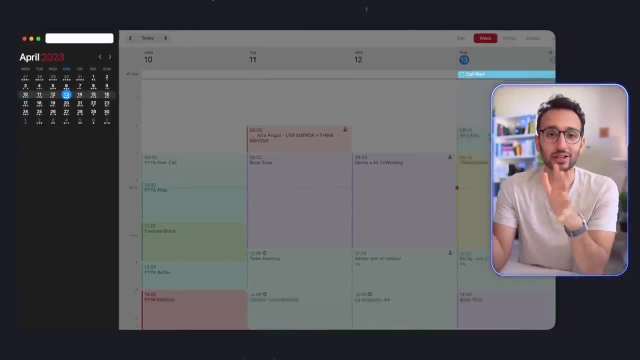 and calling my grandma is not yet in the calendar, And so I'm literally just going to add it in here as a task: Call Nani, And that will show up in my calendar. And now I know that that's going to get done because I look at my calendar multiple times a day, because my calendar tells me literally what. 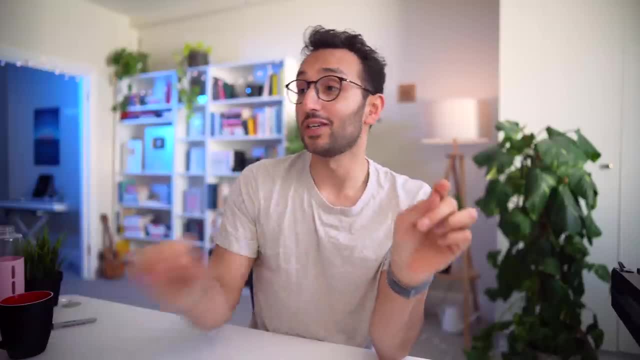 I'm doing. In fact, you know what: I'm going to be a good grandson. I'm going to call my grandma straight after filming this video And I can literally drag that task straight onto the calendar. And it's very convenient because it overlaps with the events And it means that I 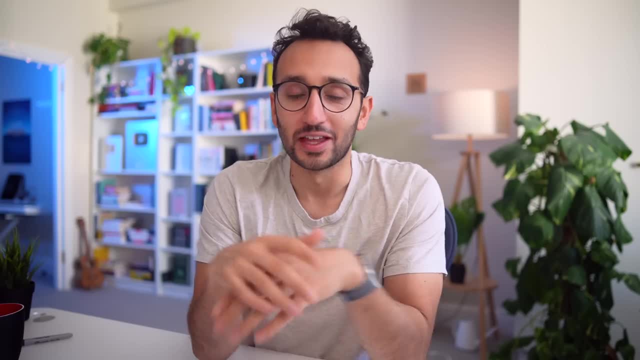 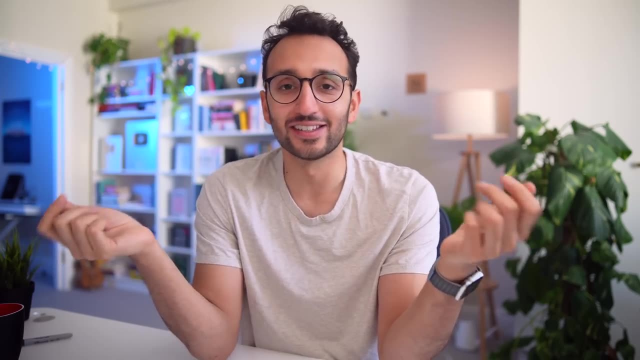 again ensure that the things that I actually want to do are in the calendar. Now, this method of like just literally running your life based on a calendar is completely game changing. I've been doing it in various forms for the last 10 years And before I started literally living my life. 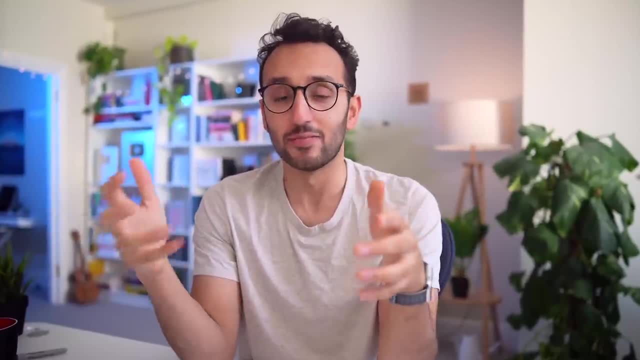 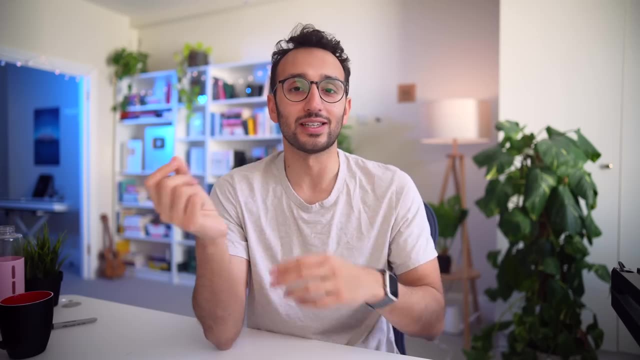 based on my calendar. I was so disorganized, I was so chaotic, But now that I live my life based on my calendar and on the level of annual, on the level of weekly and monthly and on the level of daily, I just follow the intention I've already set. That's been one of the main drivers of my 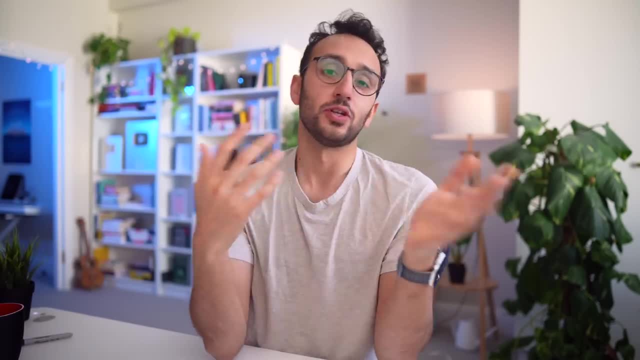 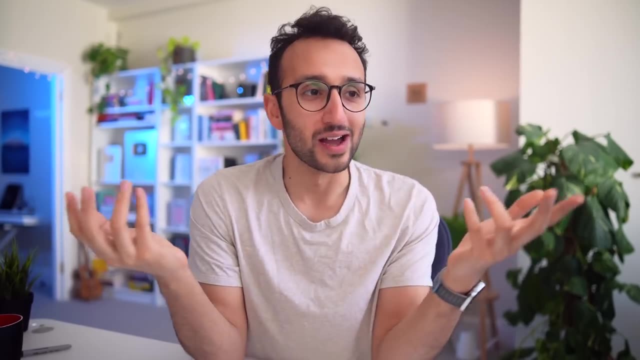 productivity for the last 10 years And specifically, this Trident method thing that I've been doing for the last eight months, since working with Eric in terms of the annual thing, the weekly thing and the daily thing, has been hugely helpful in moving me forward. And even though I'm, I think, 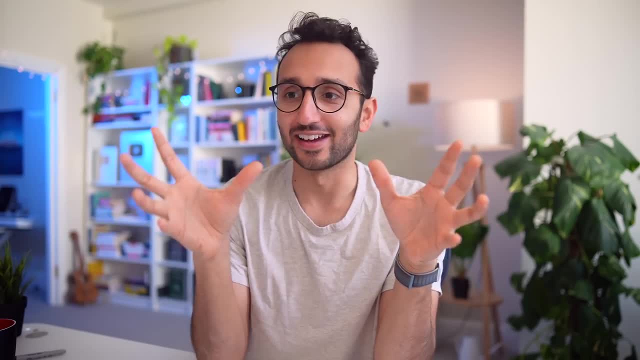 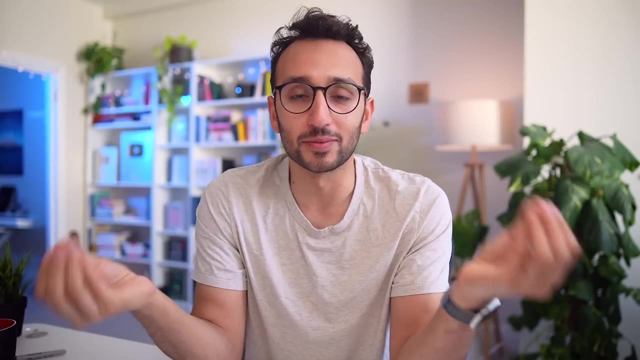 at this point, one of the most followed productivity experts in the world, like these three strategies are just have just been genuinely game changing in terms of helping me make the most of my time and helping me boost my time management skills, Because, as we've already talked about, time is the most valuable resource that we have.